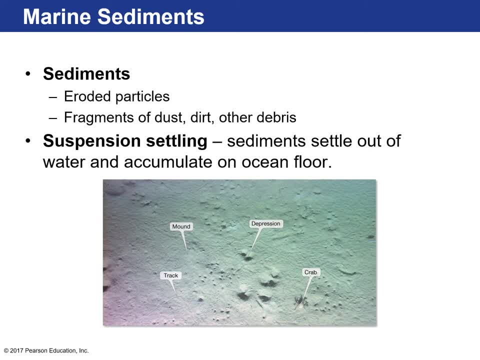 debris And they settle into the ocean floor by suspension settling. So they just kind of these small sediments, and they range in size from boulders to tiny flakes of clay and they settle out at different velocities to the bottom of the ocean floor. Larger particles settle out faster. 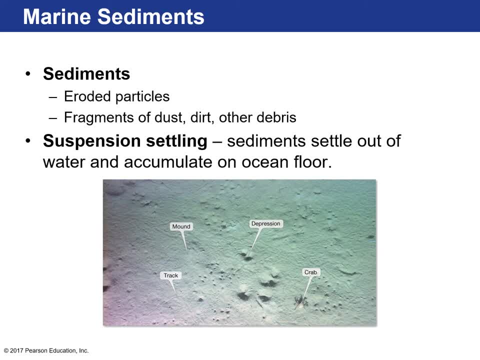 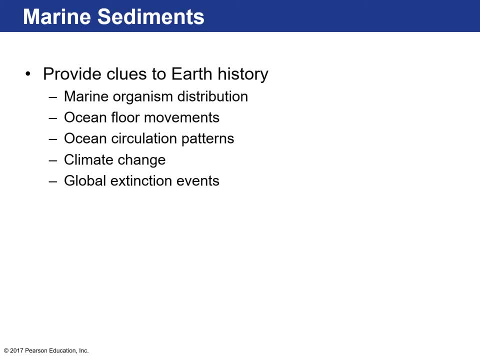 And the reason why marine sediment is so important is because it really provides a nice detailed history of our Earth that goes back hundreds of millions of years. We often find, or we almost always find, fossils of organisms, marine organisms that live in the oceans, in the water columns above where the sediment deposits, So we can understand. 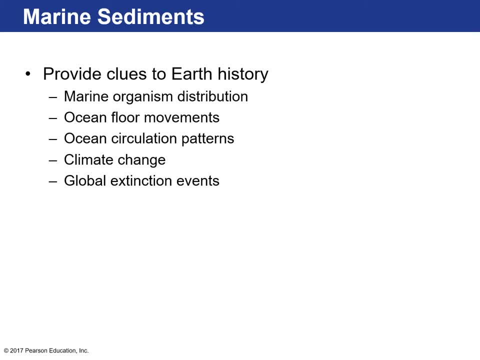 uh organism marine distribution across different parts of the ocean at different depths in different marine provinces. We can also look at the sediment history and find out when certain organisms appeared in the fossil record and we can kind of correlate that to different areas of the ocean basin. Ocean uh marine sediments also track uh ocean floor movements. 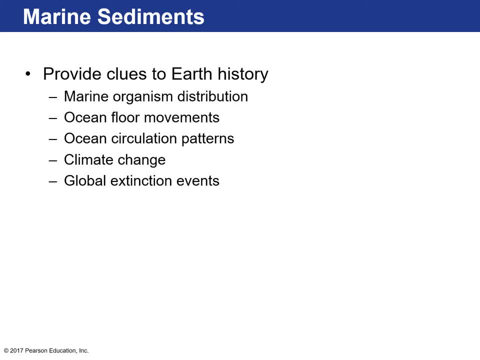 or tectonic movements, Different sediments are deposited in different marine provinces, and as lithospheric plates kind of move away, they kind of introduce the ocean floor to new environments, and so there'd be a change in sediment, so that can be tracked. 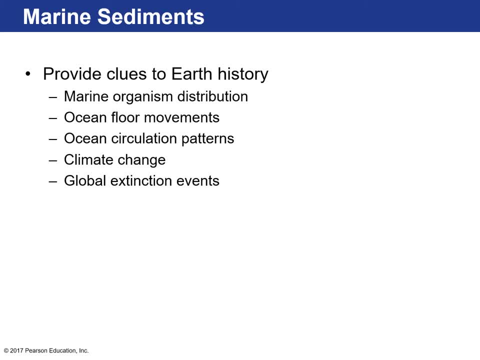 Ocean circulation patterns. there are deep ocean currents that occur uh and uh move under uh the surface, also surface currents. When those change, distribution of marine sediments can change and that can be shown in the sediment record. 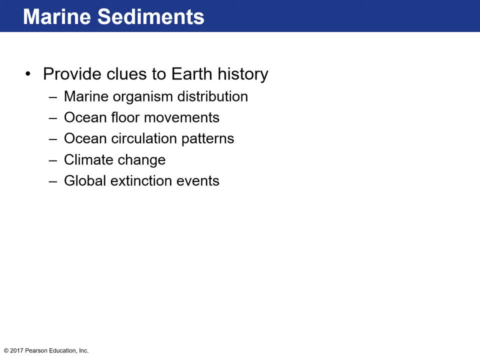 Even climate change, uh, whenever there's uh a drastic change in global climate that can change the sediments being deposited over certain marine province and that can be tracked back, And, in addition to that, global extinction events will show up in the marine sediment. 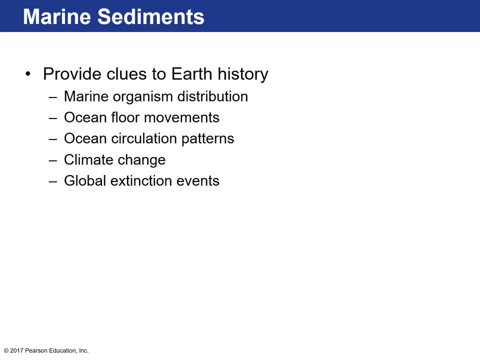 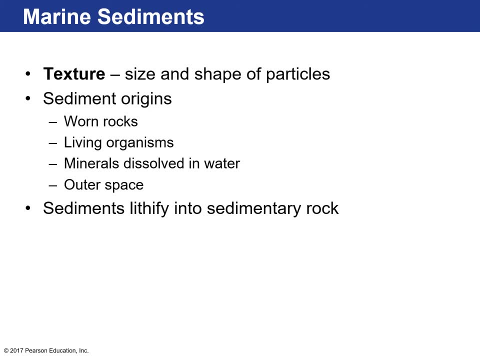 record and we can track those and compare them, how often they occur and how these or why these changes occurred. So marine sediments can be kind of divided up based on their texture, the size and shape of the particles. You can have sediment as large as gravel or boulders. 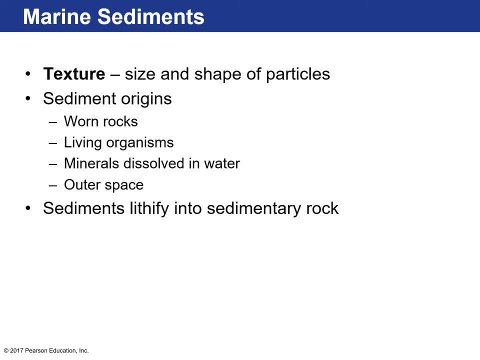 or cobbles and go all the way down to silt and clay, sand silt and clay being the smallest. Okay, also the shape of particles Sometimes, uh, sediments, um, are very sediments, are very angular, and when they're angular like that, that means they're very close to the 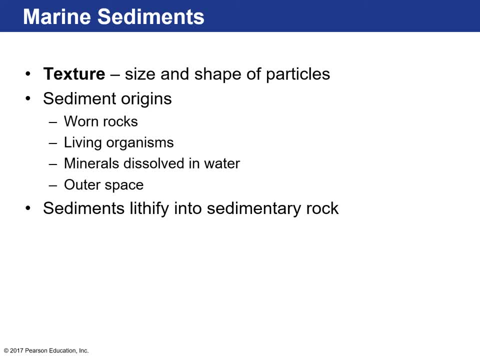 source of that sediment, meaning they haven't been worked by a lot of water. Um, sometimes you can have sediment that's very well rounded, meaning that, um, it's been pushed around by water and abraded away so that it's nice and rounded. And the origins? 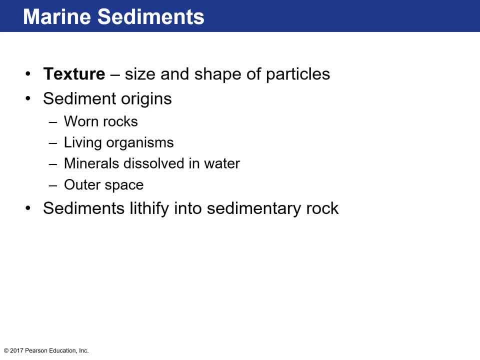 of these sediments are uh important and we can discern that uh by the different types of sediment. But most sediment uh comes from worn rocks, dust broken down, pieces that are delivered to the ocean. Uh some sediment is created by uh living organisms. 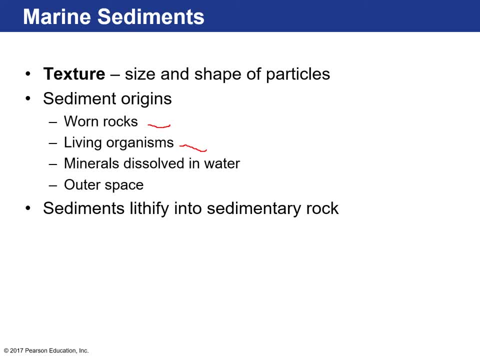 They kind of create an ornate shell kind of armor, armor, armor, armor, armor, armor, armor around themselves, Uh, and when they die, that stuff kind of sinks to the bottom of the ocean. In other, um, less frequent cases I guess it's very frequent, but in 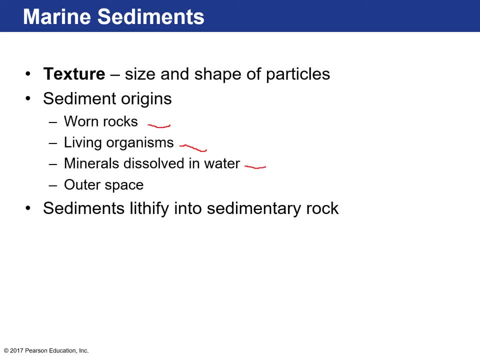 terms of volume of sediment. minerals can directly uh precipitate out of the ocean water and then deposit on the ocean floor, Um, and then a lot of space dust is delivered to Earth every year, Um, although it makes up a very small amount of total marine sediment. 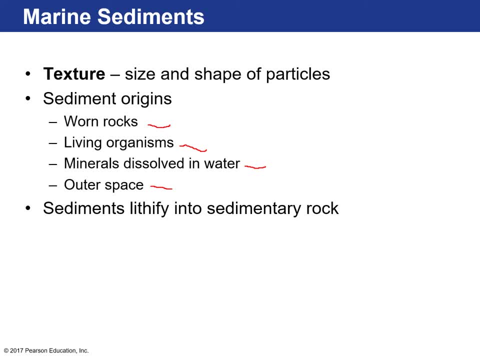 um, a lot of it is just uh microscopic dust from uh asteroid collisions or meteor, um uh meteors as they enter into the atmosphere and kind of uh vaporized and um that material can kind of slowly settle down into the bottoms of the oceans And all the sediment there's. 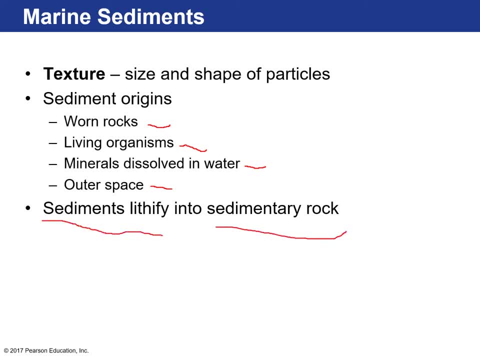 a possibility that it can lithify into a sedimentary rock, meaning that you can go from. you can go to a beach and just grab a handful of sand. That, if this, if that sand was buried on under enough pressure and enough kind of uh, water moved through it and cemented those. 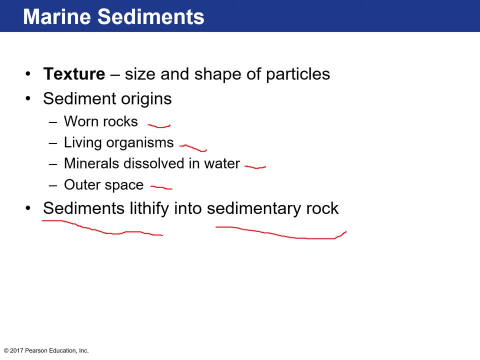 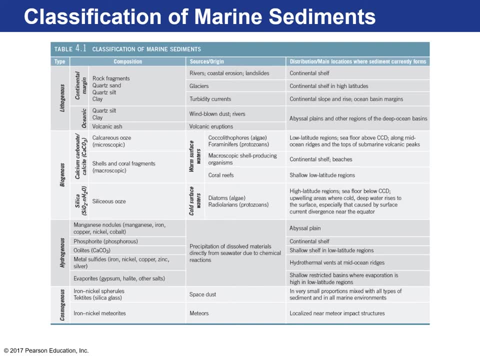 grains. together it could create a rock. That's what that means. Um and that's uh. there are a lot of sedimentary rocks found on the Earth's surface today and that's the real result of plate tectonics kind of uh pushing ocean depositional environments to the surface. 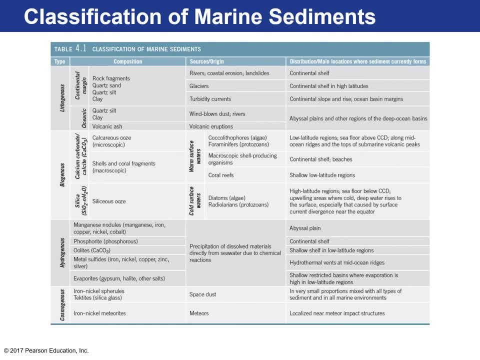 and putting those sedimentary rocks uh exposed on the surface. Here, um is a nice fancy um chart to classify different types of marine sediments. We're going to talk about all four: lithogenous, biogenous, hydrogenous. 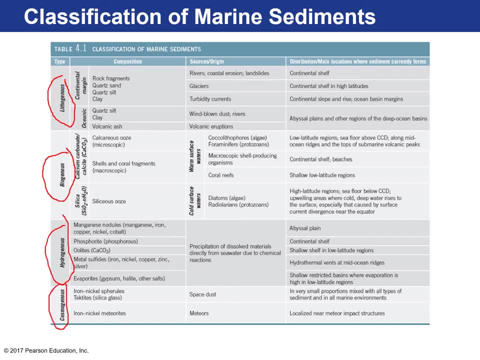 and cosmogenous. Okay, those are the four um and this is nice to reference. We're not going to go through it all, but just to reference what each one of those categories of marine sediments are composed of, where they come from, okay, and their distribution in the 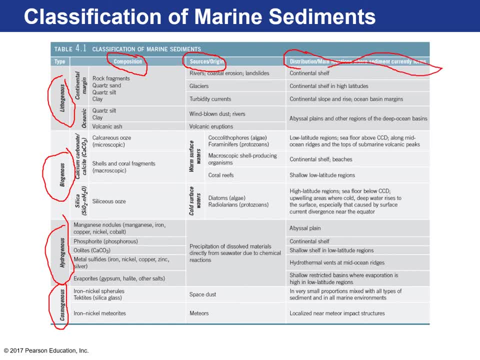 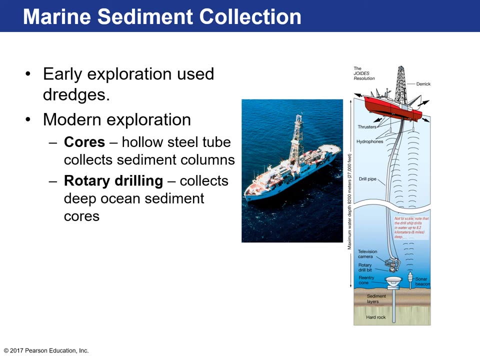 different marine provinces. Okay, So you can uh go back and reference this, Um maybe download the PowerPoint and that'll help you understand the different types of uh marine sediment. And, over time, uh humans have collected marine sediments in a number of different ways. Uh, the most classic way was just dredging. 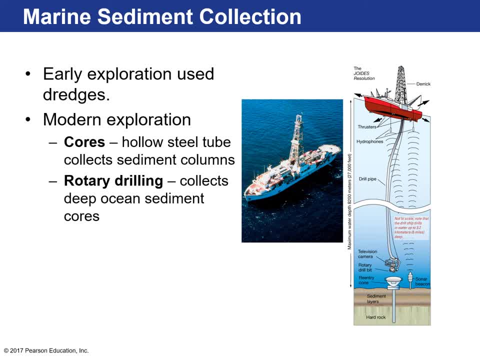 which means just throwing some sort of mechanism overboard and just grasping the bottom of the ocean floor and grabbing as much sediment as you possibly can. Uh, very crude. Um, it disturbs the sediment. Um, it really is. you can only really find out what's on the surface of the. 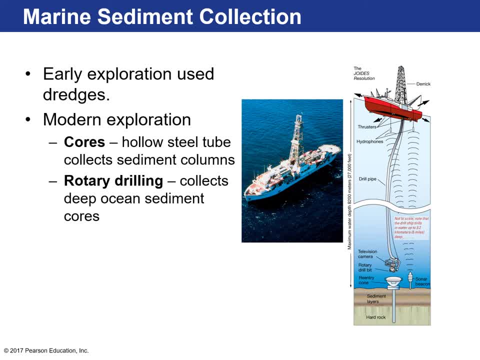 ocean floor. Uh, so not super useful. but later on, uh, our modern exploration, we started to drill cores, And what cores are are just, uh, hollow steel tubes that are pounded into the ocean floor. Okay, So here is a cross section. Okay, It's not the scale, but here 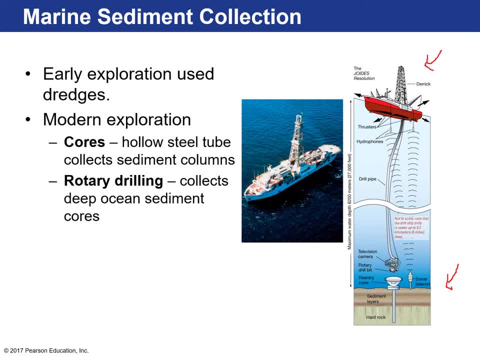 are the kind of modern ships, Drill drilling ships, which is pretty crazy. they have thrusters to kind of keep them steady. but then there's this, these steel hollow drill pipes that are all connected together and co can. now, today's technology can get down to um, uh, over seven kilometers, um, and then 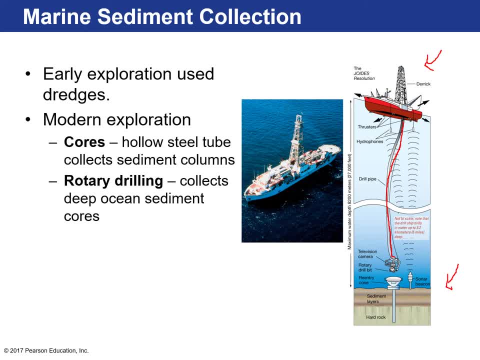 uh, they go down into this um re-entry cone and then right down here is a rotary drill bit and that breaks up the rock all around um the well. it breaks up the sediment and then all the surrounding hard rock once you get to the hard rock. but it brings up. 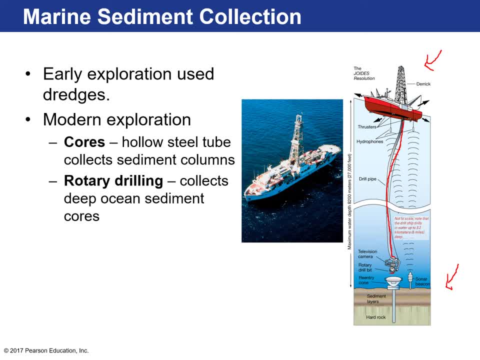 a cylinder tube or a core sample up to the surface and onto the boat where you collect that information. okay, and that that has been the kind of major advances in collecting deep sea sediment and also collecting it kind of in the order that it was deposited, which is very useful in understanding. 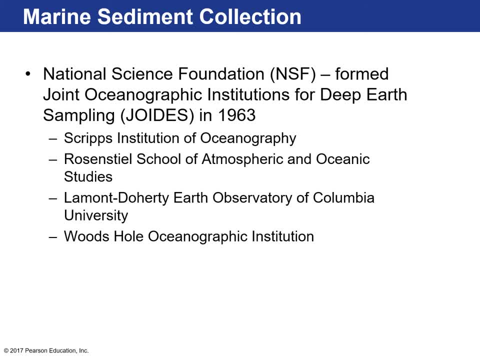 uh, things that have occurred in earth's past. so the national science foundation really started this. this agency started this project in 1963- the joint oceanographic institutions for deep earth sampling- and it included three major schools of for oceanography. if you're interested in majoring and then doing research or work in anything, 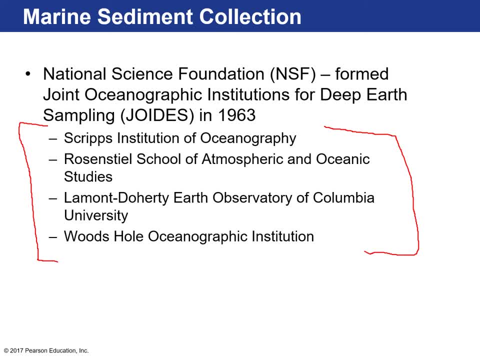 that has to do with oceanography and earth science. uh, these are great places: scripps in san diego, the resential uh school of atmospheric and oceanographic studies that's in miami, uh lamont doherty at columbia university and uh woods hole. okay, so they developed the. 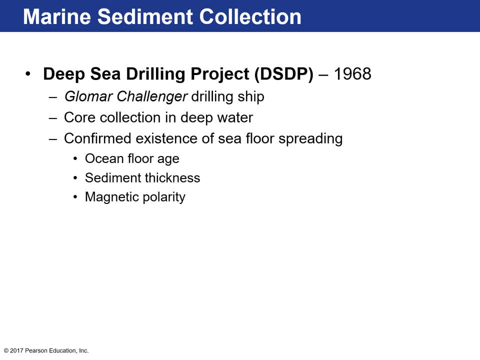 that agency, in partnership with those institutions, developed the deep sea drilling project in 1968 and the glomar challenger was the drilling project and they had over- i think it's over- 200 different cores and different parts of all the ocean basins and they found out a lot of information, in fact. 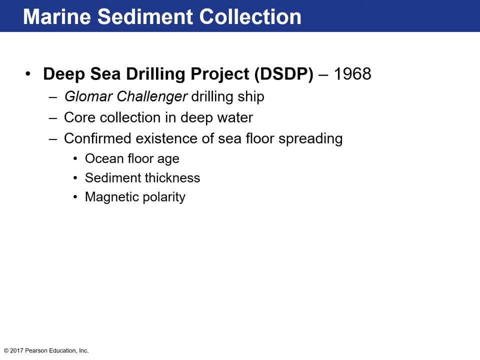 they confirmed the existence of seafloor spreading. so back when we talked about plate tectonics and the evidence that supported plate tectonics, part of these expeditions helped kind of cement that paradigm shift with the introduction of plate tectonics theory. so one was 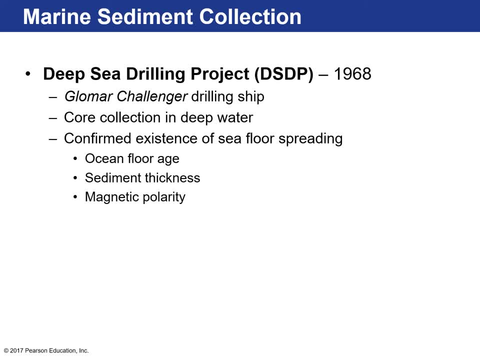 um. they were able to drill down through the sediment and get down to the hard rock, and the hard rock is basalt. that's the ocean floor rock, and you can age date that. and so what they found was ocean floor age um increased as you go away from the mid-ocean ridge. 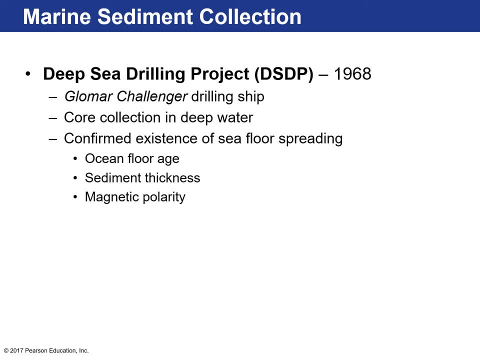 and as you get closer to the mid-ocean ridge and into the rift valley, that's where you find the youngest ocean floor rocks, and so that kind of confirmed that new, new ocean crest is being created at mid-ocean ridges and then it spreads outwards in addition to that sediment. 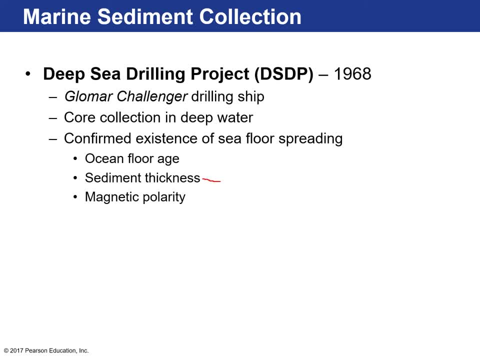 10. the thickness of sediment above the hard basaltic rock in the ocean was thicker the further you go away from the mid-ocean ridges, which makes sense because if they're older rocks, they've been at the bottom of the ocean for longer and allows for more time for this. 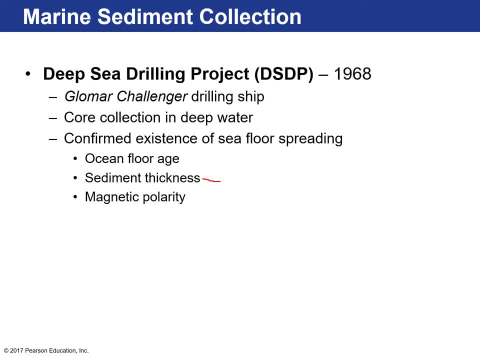 dusting of microscopic marine sediment to kind of fall on top of that hard rock. and then, in addition to that, they found the kind of basically the mirror image, in terms of magnetic polarity, in those basaltic volcanic rocks at the bottom of the ocean on either side of the mid-ocean ridge. 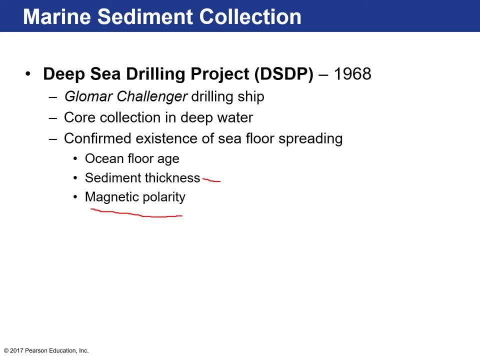 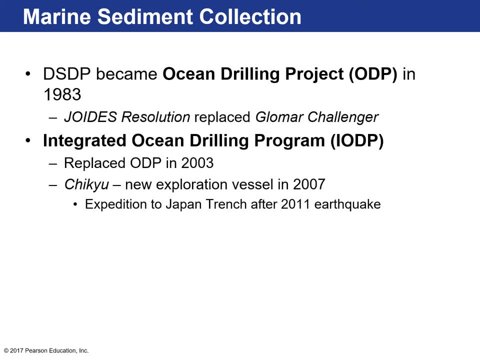 and that really is what, um this? this was the smoking gun that that helped, uh, support the theory of plate tectonics and sea floor spreading. okay, later on, the ds, the, the deep sea drilling project, became the ocean drilling project in 1983. glomar was the, the ship itself was replaced and then it became the integrated ocean drilling. 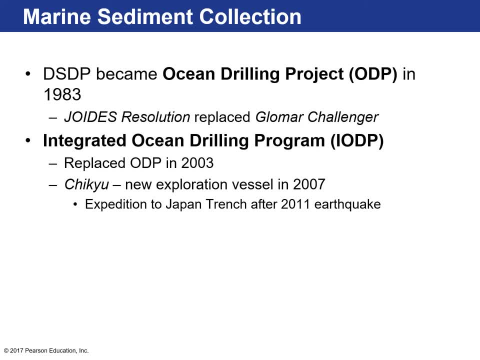 program. a number of different countries were invited to participate and, um you know, pull up their resources, and the odp was. the odp was replaced in 2003 and new ships have been added. the cheek u is uh kind of a newer vessel, built in 2007. 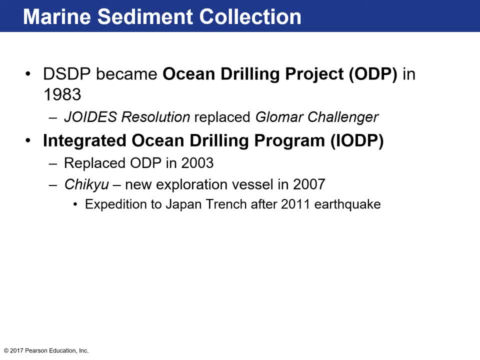 with the most uh updated technology can drill the farthest. in fact, it went to the japan trench after the tohoku earthquake in 2011.. so this is an ongoing. this is where the real ocean uh science is. this is like the frontier of new research, or from these drilling programs. 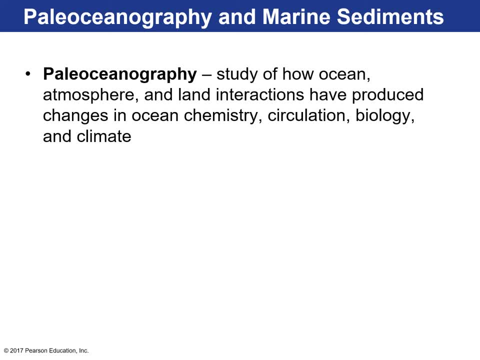 and the science that unders or uses marine uh sediments to kind of understand how the ocean or atmosphere and land interactions have changed the ocean chemistry or any ocean circulation or any organisms or climate associated with. that is paleo oceanography, and here's an example of what a core looks like when you bring it to the surface. 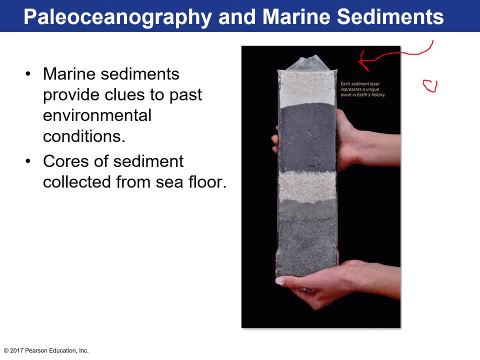 okay, now it's it's. they're cylindrical shaped, okay, so the cores come out like this: okay, i'm a terrible, that's a cylinder, but they're cut in half, and so this is one that's cut in half, and then you can see here what's on top would be the youngest sediment, okay. so just imagine, this is the ocean floor surface. 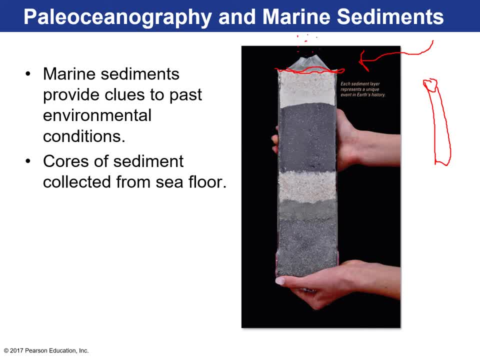 a new sediment kind of suspension settles from the water onto the surface of the ocean floor here. so these are the youngest sediments and so then you can assume down here are the oldest sediments. so this represents an interval in time in earth history where sediment has been accumulating in this particular sediment. 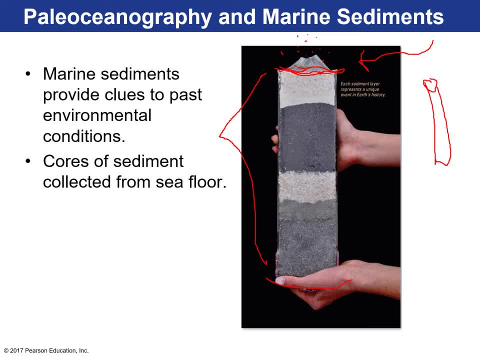 in this particular sediment, in this particular area, wherever you drilled for it, and so the reason why marine sediments are important is because you can clearly see. do you see these changes? you can see changes in texture, color. if you looked in more detail, i'm sure you'd find differences in marine organisms. 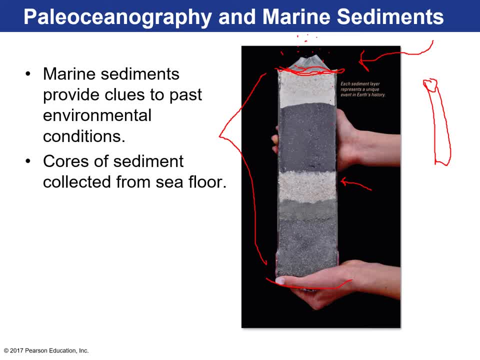 microfossils that you'd find. so perhaps right here, this material here looks a little coarser, more gra, filled with gravel. perhaps sea level fell and the environment changed and now this was closer to the continents, so larger particles of sediment began to deposit here much more recent times, or something okay, and then here this looks like more clay. 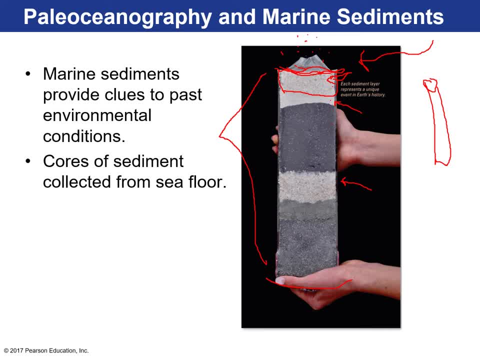 perhaps more biogenous sediment, organic in origin, so there might be salacious or calcareous oozes found here, who knows. and then maybe here you'll find a layer where there's a lot of- uh, very fine volcanic ash or something like that, and that would mark. 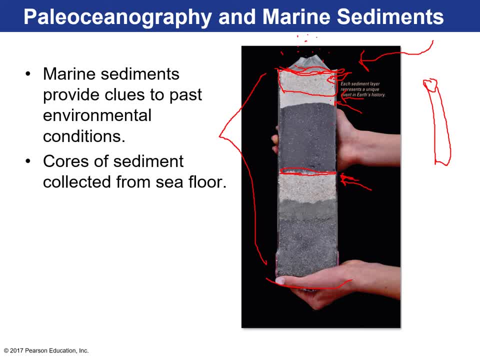 a volcanic eruption in the nearby area, okay, or you'll find some cosmogonous sediment that have extra extraterrestrial in origin. it might record a global extinction event. so these are the reasons why marine sediment is important, because it kind of provides an uninterrupted history of our earth. 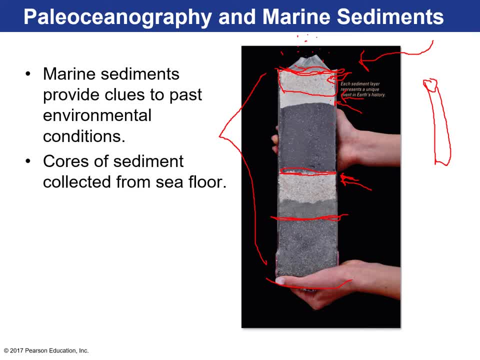 as recorded by sediment in the oceans. and here's an example of two scientists working with cores that were just pulled up on a ship. and here's an example of two scientists working with cores that were just pulled up on a ship. and here's an example of two scientists working with cores that were just pulled up on a ship. 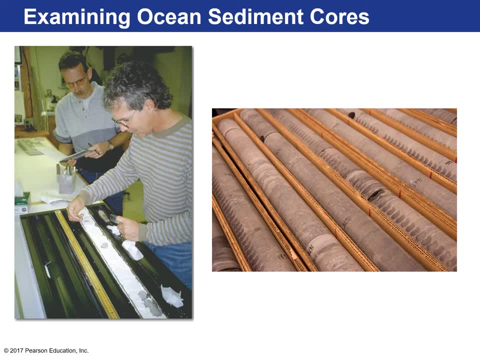 you can see here. this is the cylindrical shape of them. okay, these are the cores pulled up. they're all numbered, different intervals top to bottom, so we get a good idea of what occurred first, what occurred afterwards, and then we put specific time markers for certain events on them. 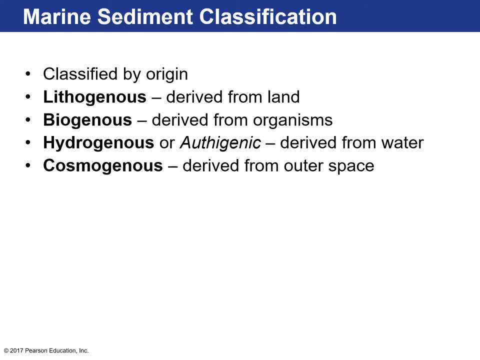 all right. so the way we classify marine sediment is based on these four types, which are classified based on their origin: lithogenous sediments that are present in the oceans, and we're going to go through them now. the anybody can guess what sediment is. it's technology. 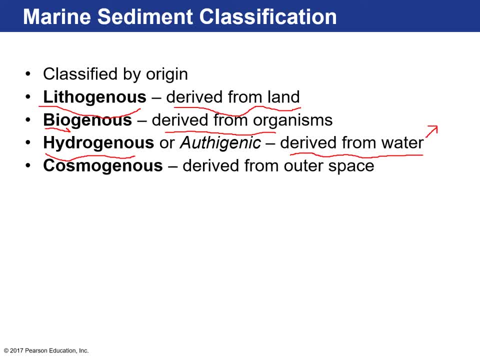 because, with chemistry, certain dissolved solids may increase in concentration high enough to the point where they start precipitating out of the water and deposit on the ocean floor. And then cosmogonous: those are sediments that are derived from outer space. Okay, so let's go over lithogonous sediments. These are 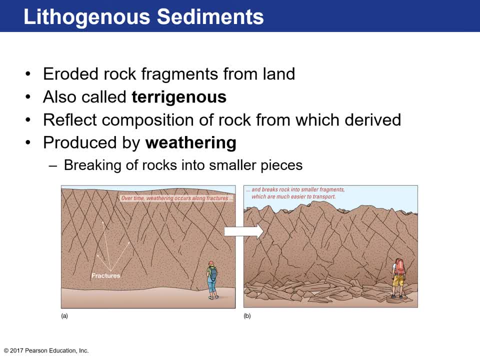 just eroded rock fragments from land. They're also called pterygionous because terra is kind of like Latin root word for earth. Okay, the the different types of pterygionous sediment really reflect the composition of the rocks that are. 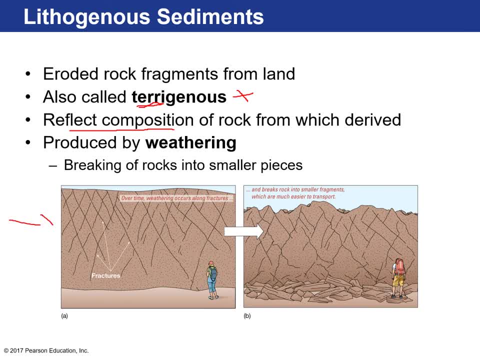 eroding on land. So let's say you have a rock here. over time you get fractures and joints because of differences in pressure, There's weathering that occurs and then these rocks are fracturing at this point and there's still a lot of. 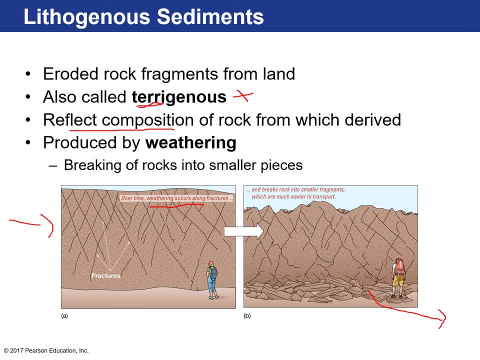 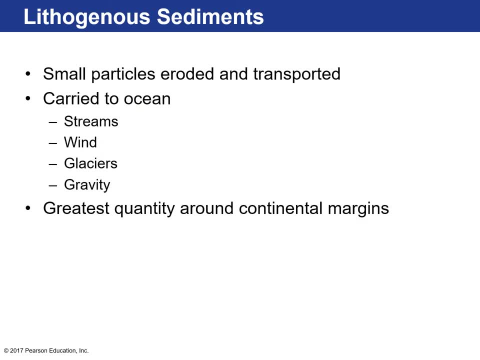 smaller pieces and that stuff eventually can be moved down into the ocean. So rocks tend to break down into smaller, smaller pieces And then under the force of gravity, wind or even water, they kind of help travel down to the oceans. 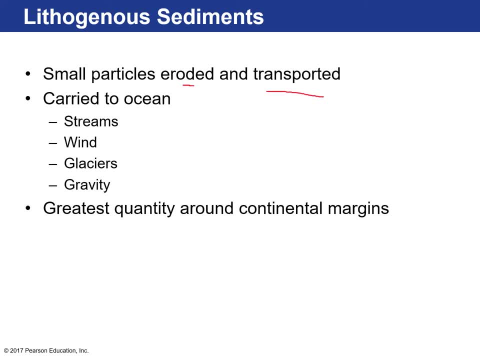 So these small particles erode and then are transported. They're carried to the ocean from streams, wind, glaciers and gravity. So the greatest quantity of lithogenous sediments are around continental margins, which makes sense, because continental margins are areas that are next to the continent. 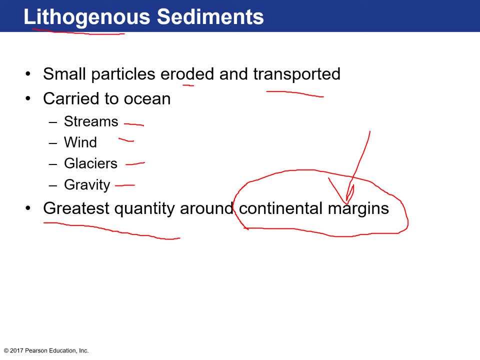 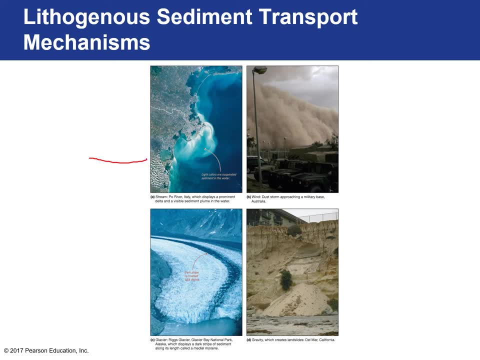 And if you have sediment that's derived from rocks, from the continent, of course, the greatest quantity would be closest to those continents. So here's some cool examples. This is the Po River in northern Italy. You can see the river dumps out into the Mediterranean Sea here. 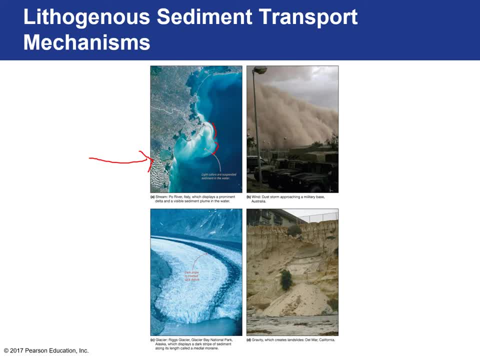 And you see this plume of rock, Very light sediment, kind of changing the color of the water. That's all sediment that's in suspension, being delivered into the ocean. Eventually it'll settle and deposit out on the bottom of the ocean floor. 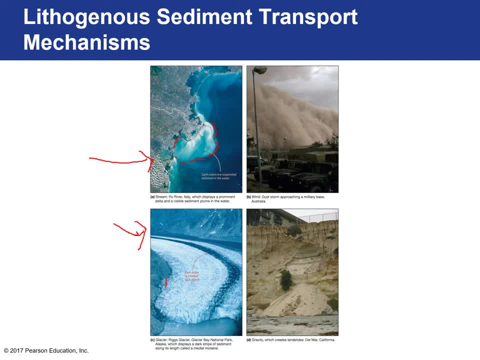 Glaciers. they do a lot of work actually. They grind rock kind of underneath the glacier here and then that kind of pushes a big, like bulldozes, a big amount of sediment directly into lakes or into the ocean. But also there's here these moraines in the middle. 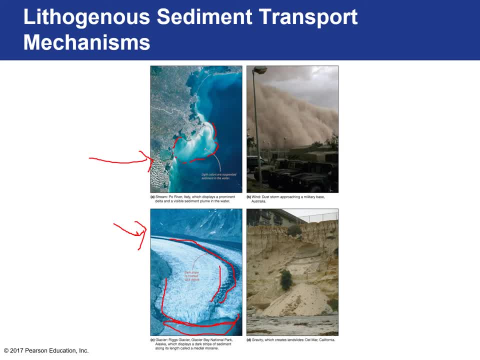 And you can see that there's a lot of sediment. You can see that there's a lot of sediment in the middle of a glacier that are covered by sediment, And a lot of sediment gets kind of piggybacked on top of the glacier and then delivered to. 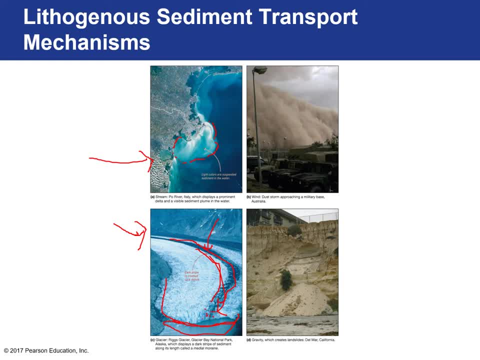 the ocean, Or there's sediment that's inside the glacier, inside the ice, And as the icebergs kind of break off and calve into the ocean, they slowly melt and then they drop their sediment load. Okay, And if you've been to anywhere that's really dry, where there are deserts, you can often 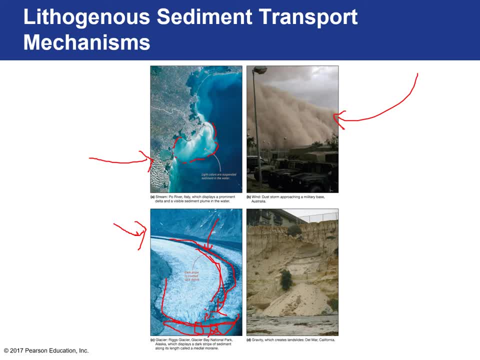 get sandstorms like this And wind can pick up really small particles and then blow that right over into the ocean And then in places like California you can have cliffs by the ocean and then you just get gravity pulling down on this material as it kind of mass wastes close to the ocean. 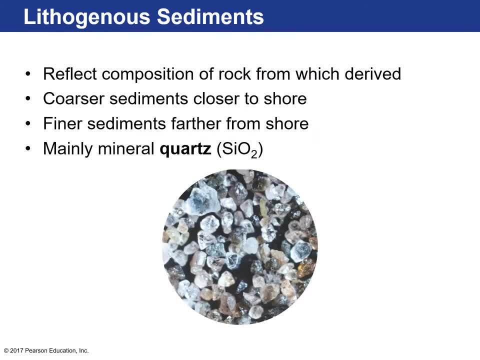 floor and then it can fall into those breaking waves. So that's how they get transported. So the composition of lithogenous sediment reflects the rocks that are close by. Coarser sediment is closer to shore, Meaning that like they're closer to the shore, 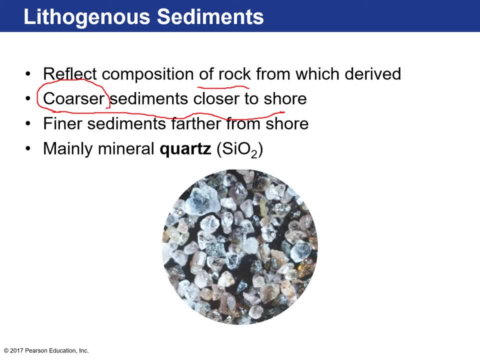 Closer to their source. They haven't been worked by water and smoothed out. Finer sediment is typically found further away from shore, And that's because coarser sediment is heavier, has a faster settling velocity, So they'll deposit out really quickly. 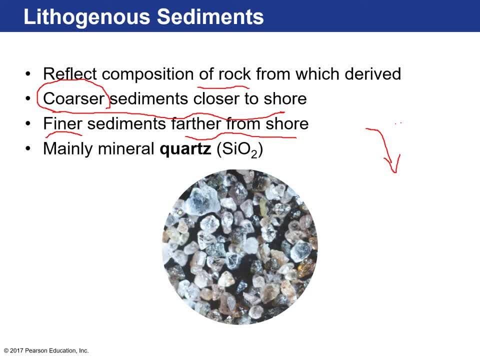 Fine sediment will remain in suspension in the water for longer because their settling velocities are much slower. Okay, And one of the most resilient minerals in rocks is quartz. They're resilient to weathering, So a lot of lithogenous sediment. It's composition is actually quartz SiO2, which is pictured here. 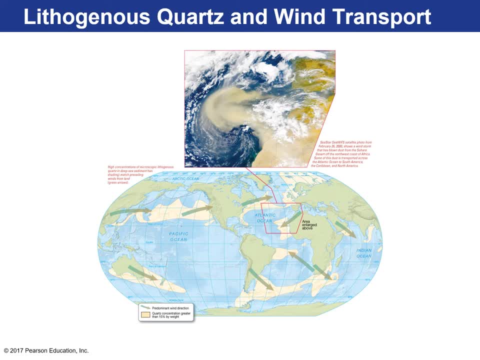 Here's an example of lithogenous dust from the Saharan desert being delivered to the Atlantic Ocean via the global wind belts. okay, So here is the Saharan desert. okay, We have the trade winds that are persistent winds that blow over the African continent. 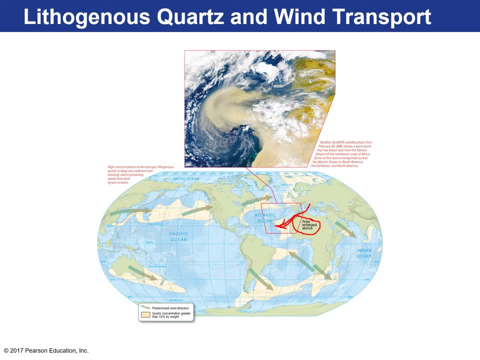 And it blows a lot of Saharan dust into the desert. Okay, So here is the Saharan desert. Here's a lot of lithogenous sediment being taken out into the Atlantic Ocean. So we see a lot of lithogenous, very fine sediment being blown up and taken into the 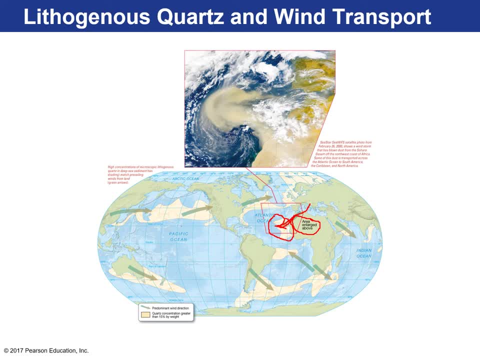 atmosphere and deposited out into the Atlantic Ocean. Sometimes these plumes make it all the way to the Caribbean and even into Florida. That can cause kind of allergic reactions to some peoplemight have adverse reactions to that. It also makes the sunsets and sunrises a little pinker and hazier. 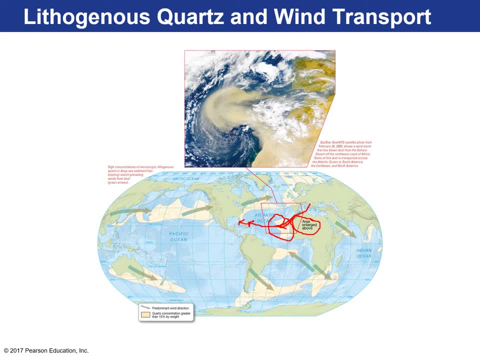 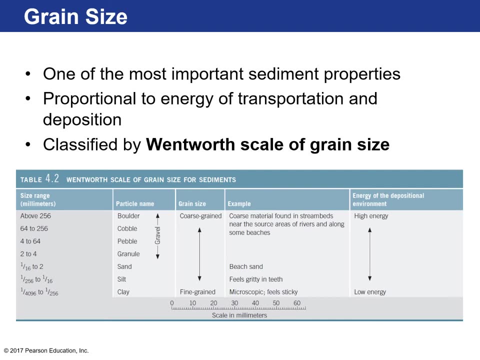 All right. So here's a little bit of the Saharan desert. Here's a little bit of the Saharan desert. okay, here's the Wentworth scale of grain size. I've talked about this. this is how we classify different sizes of sediment. okay, largest being Boulder. okay, smallest being clay. so whenever I 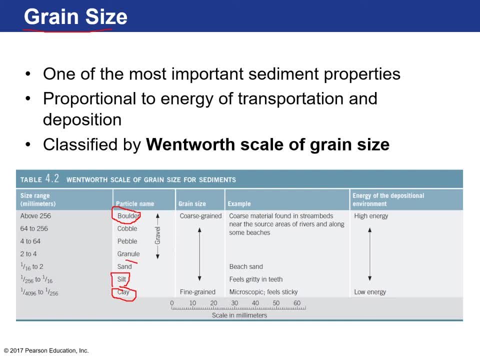 ever say small clay. clay and silt are the smallest. then there's sand, granules and pebbles. here's the size range in terms of millimeters. okay, so sand would be anywhere between 1 16th to 2 millimeters in size. all right, so just to get an idea, anything that's larger is considered coarse grained, and 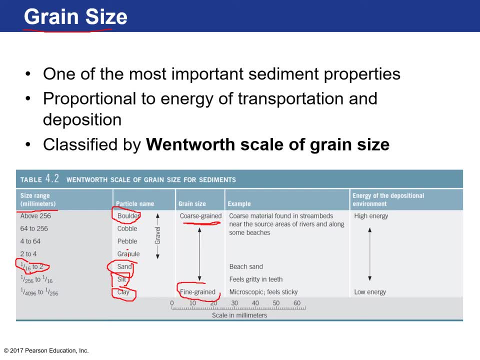 anything that's small, like silt or clays, well, is what we call fine grained. so beach sand is typically sand sized stuff: microscopic, soft feeling, sticky feeling, kind of muddy stuff would be more like clay, okay, and then the sediment indicates the depositional environment in which it was. 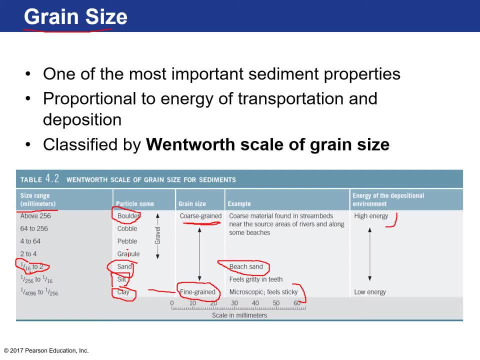 deposited. so larger grained sediment typically are deposited in high-energy environments, think of like where the waves crash on the beach. that's typically where you find your largest pieces of sediment that are piled up because they're- you know, because they're kind of high-energy waves. 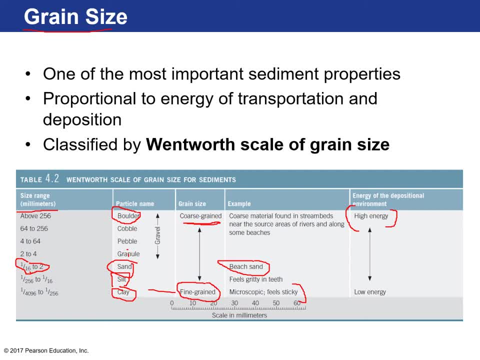 crashing down and that kind of picks up heavier sediment or larger sediment, lower energy environments let's think of like a lagoon or something like that. those are really low energy. then you'll find a lot of that allows for the really small particles the settle out and deposit. so bays and muddy areas, lagoons and 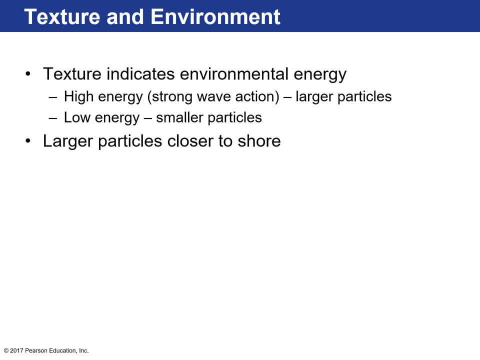 stuff like that are considered low energy. so the texture of the sediment that you find can indicate the environmental energy: high energy, strong wave action, larger particles. if you have a low energy environment, that means smaller particles and typically larger particles are closer to shore and that's because they deposit out quicker, because they're heavier. 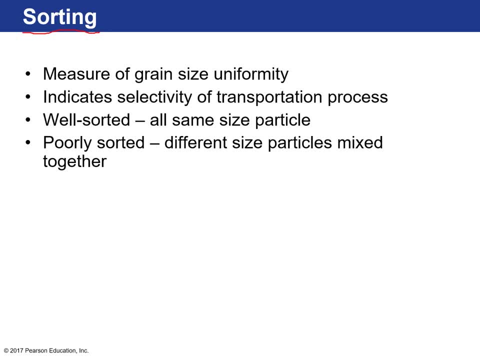 sorting is a dis, a way of describing um the grain size uniformity, meaning that, like if you have a bunch of marine sediments that are all the exact same size, that means that that is well sorted. um, if you have a lot of marine sediment that consists of boulders, gravel, clay, sand and a bunch 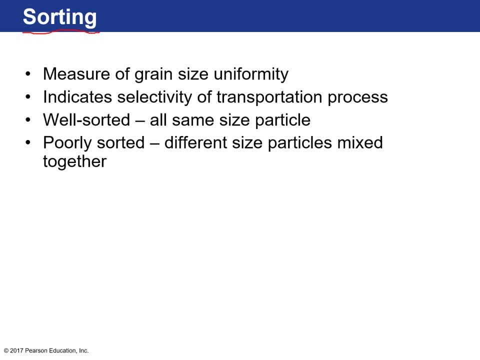 of different sediments of different sizes. we would consider that poorly sorted okay and that's indicative of the type of environment it can come from: typically well sorted deposits, something like wind deposit- wind deposits because wind can only pick up a certain size sediment, clay, silt and 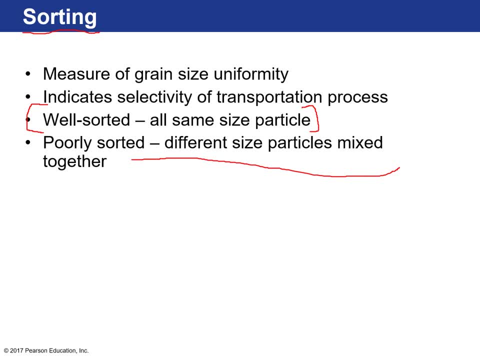 maybe the finest sand right. so wherever that deposits out from the wind, that depositional area is going to have well sorted sediment, because wind can only carry small particles so all those will have grain size uniformity. okay, if you have a major landslide or a massive turbidity current which is an underwater, 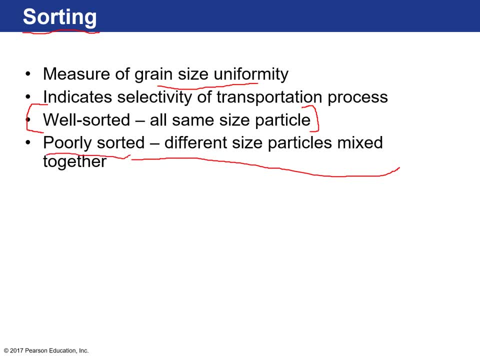 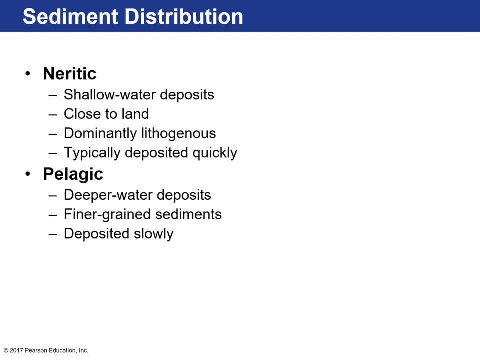 landslide. you're going to have poorly sorted sediment as a result, because those are kind of high energy kind of pick up all the different size sediment and deposit them all together. so how is sediment distribute? distributed? there are two major environments: the neuritic environment, which translates to shallow water deposits very close to land. 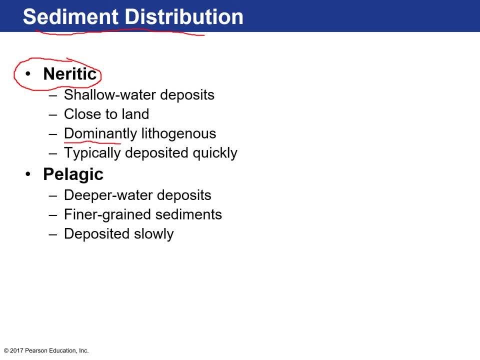 neuritic environments. most sediment found here is lithogenous and that makes sense because they're close to land and these sediments typically deposit quickly- delivered from rivers or some other source, directly into the water and they deposit out very quickly. it's really passed down дніrosเลย. 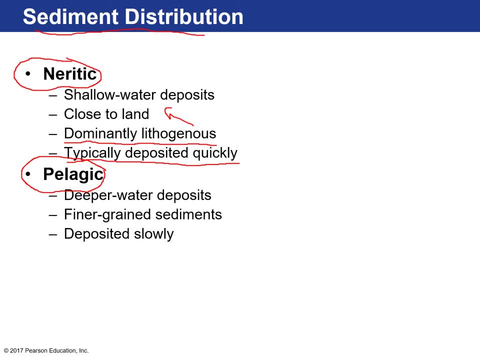 to abyssal, through water, through the abyssals, a blast of sediment, get acid. you know you really want to get some great sediment. so other agents in a watershed may have their hairstyle their. they make it to the bottom of the ocean and that's a combination of the, the deep, 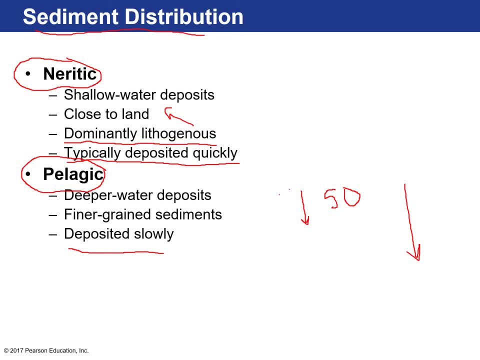 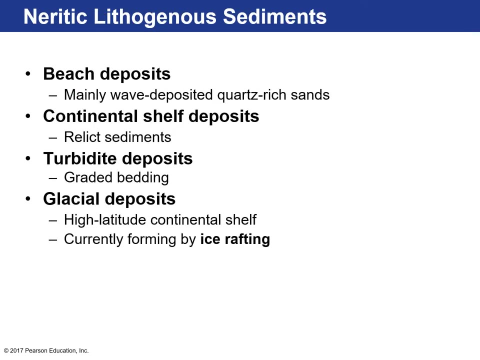 waters of the ocean. it's very deep, yes, the traverse on average about three and a half miles, but there's seven. settling velocities are so slow, so that's why it takes so long. okay, so let's talk about some of the neuritic lithogenous sediments we have: deep beach deposits. these are the ones that you're probably 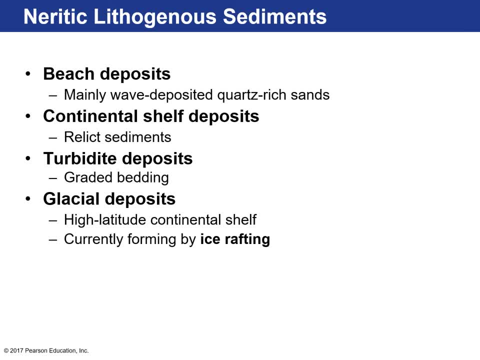 most familiar with these are wave deposited, usually quartz rich sands. quartz quartz is kind of colorless or even white. so that's where you get those kind of white sand beaches from continental shelf deposits. these are deposits and kind of deeper deposits than beach deposits out on the 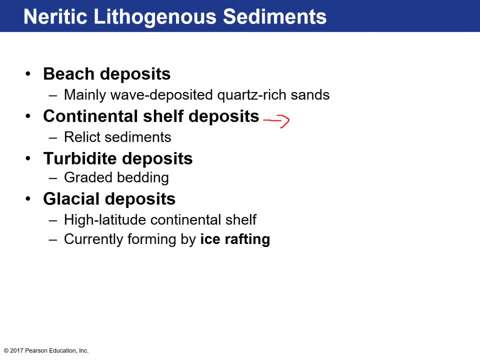 continental shelf and that's mainly finer stuff in comparison to the beach deposits, but still kind of large inhaling lie. so you know it's. it's much larger lithogenous material than you'd see on the pelagic environments. sea level fluctuates goes higher and lower. 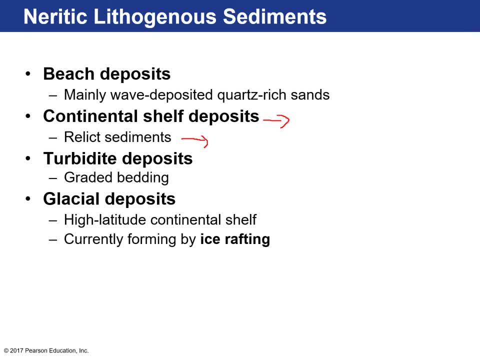 during our last glacial period. our last glacial maximum was about 18,000 years ago, but pretty much the the cooler times about 10,000 years ago. and when earth is much cooler, there's a lot more water in the form of glaciers, continental glaciers on land, so that lower level is much more. 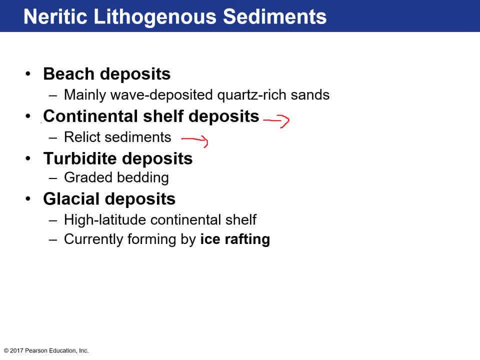 sea level. so a lot of our continental shelf during our last glacial maximum was exposed, and so a lot of the the rivers that empty out at the sea today actually deposited a lot of sediment on these continental shelves, and that sediment we refer to as relic sediment, because there's sediment that was. 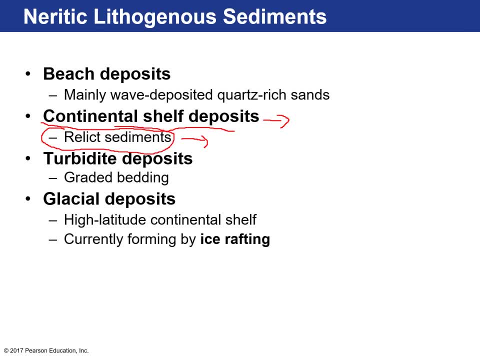 deposited there as a as a relic of the last cooler time period in Earth's history. there and then there are turbidite deposits. these are underwater landslides that occur along the continental slope. these are kind of muddy mixed waters that move quickly downhill under the force of gravity. that 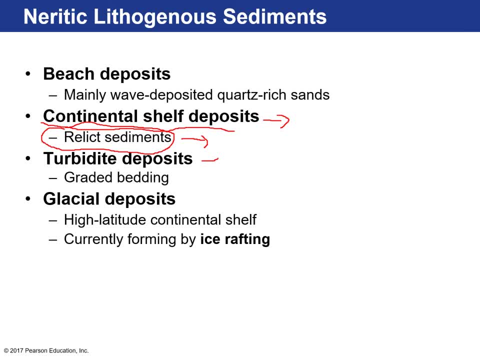 carry a lot of different sized particles and they leave graded bedding deposits. okay, then there are glacial deposits, and we see these really in high-latitude deposits and we see these really in high-latitude areas that are close to the ocean and on the continental shelf, and a lot of the 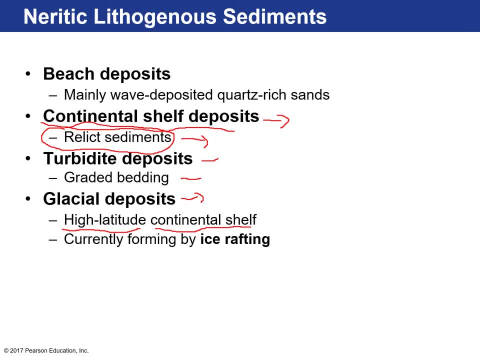 sediment kind of can get bulldozed from glaciers, that kind of calve off into bays and into oceans. but a lot of times they calve off giant chunks of of ice into the water and they get swept up by ocean currents. but within those big 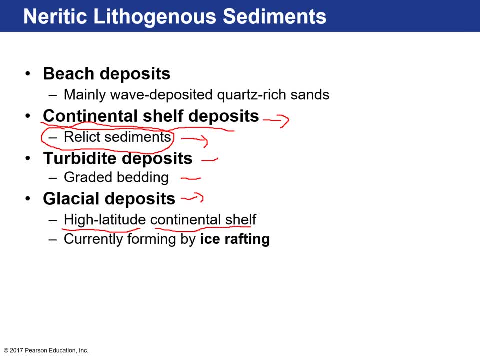 chunks of ice. those icebergs, they have a lot of trapped sediment and so that those icebergs- all right, those are the icebergs that are in the middle of the ocean, and these are the icebergs that are in the middle of the ocean, and these are the 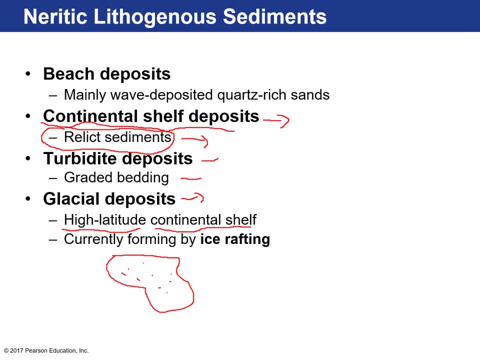 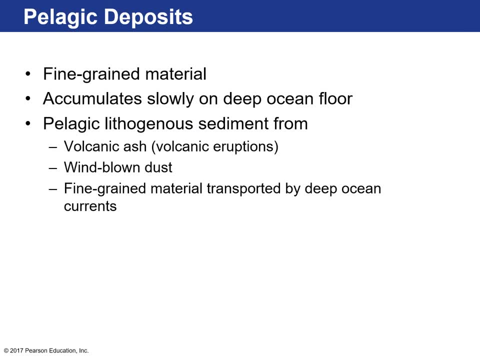 icebergs that are in the middle of the ocean, and these are. the iceberg has a lot of trapped sediment in it and as as the iceberg melts, then the sediment will be dropped from those icebergs, gullet ice, rafting in pelagic settings, way on the 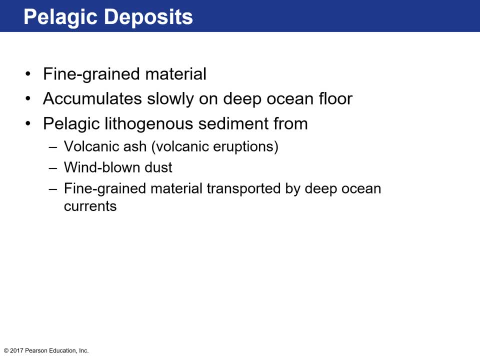 deep ocean we typically find very fine-grain marine sediment. okay, it accumulates very slowly. in the deep ocean. these sedimentation rates, or accumulation rates of marine sediment, can be millimeters per thousand years, and theonto takes a lot of energy to get out the sediment that it is to return. so 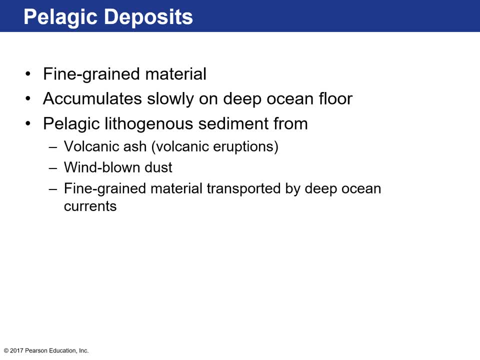 it's very slow, and so a lot of the source of this pelagic fine-grained material is volcanic ash from eruptions, windblown dust like from the seren desert like we talked about, or just really fine grain material that was delivered to the ocean and just slowly settling out alright, and so in those 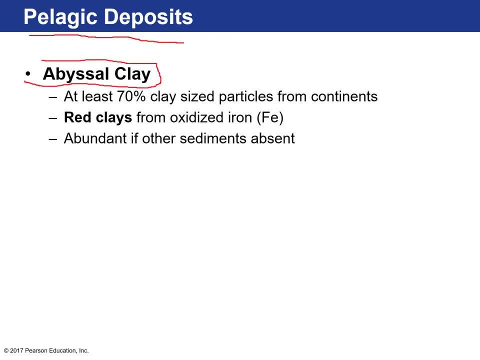 works is abyssal clay? okay, because it's. the definition is that it's at least 70% clay sized particles from the continents and a lot of times abyssal clays. they're called red clays and the reason is is because that they often have a lot of. 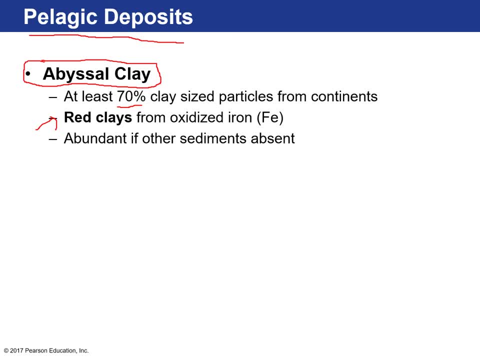 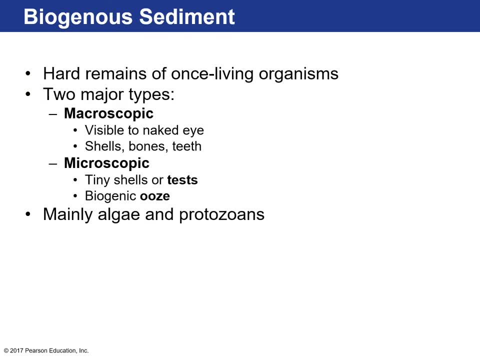 oxidized iron in it and that gives them that kind of red color. okay, now let's move on to biogenous sediment. biogenous sediment is made up of hard remains of once living organisms, and there's two major types. there's macroscopic and microscopic. macroscopic is something that you can see with the naked eye. you 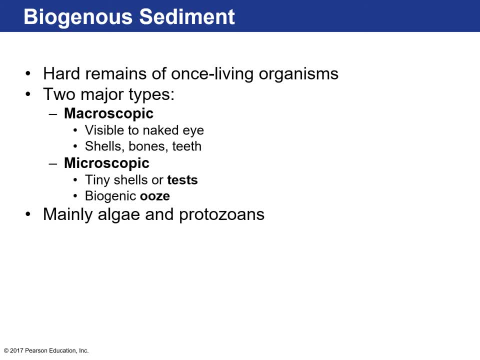 can just say: you're walking on a beach and you see some shells, bones or any teeth that are. those are remains of organisms that were living like. if you go to Lido Key, which is off the it's on a barrier island near Sarasota, it's chock-full of. 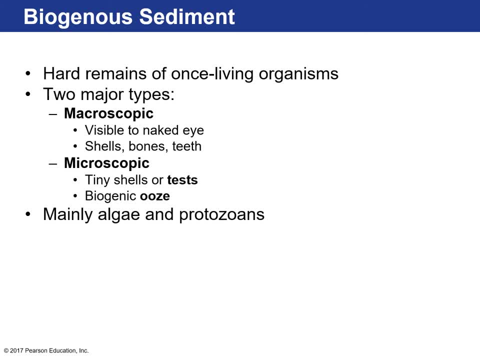 macroscopic biogenous sediment all washed up by the waves, okay, but that doesn't make up a lot of the biogenous sediment. those, those environments are actually quite small in comparison to the deep ocean. in the deep ocean there's a lot of microscopic life that floats around the sun little. 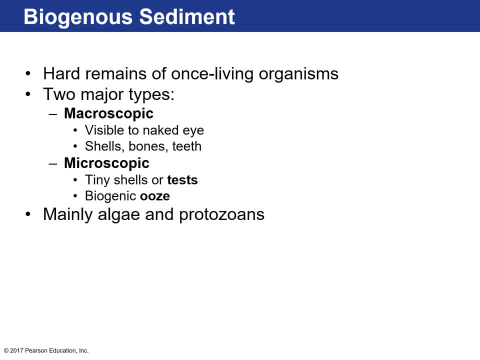 layers in the deep ocean and those organisms. they create really tiny shells and we call them tests or shells, and the when they die they may live a couple days or a week. when they die, those shells kind of rain down to the bottom of the ocean floor and they start creating a type of sediment called by a. 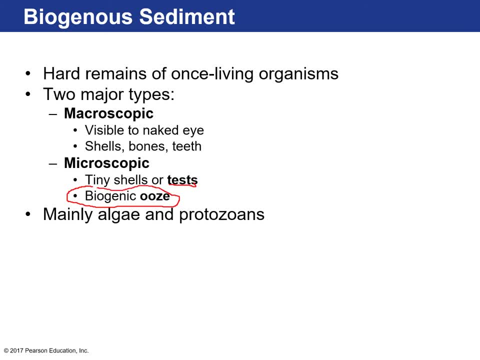 biogenic ooze. okay, the reason why it's called the news is because it's think of like, say, you have toothpaste and you squeeze some of it out and you mix it with water and then you just kind of mix it in. it's kind of very soft, kind of. 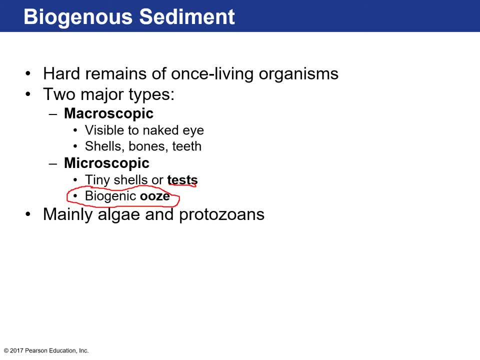 water mixed material with very like clay type soft material. so the reason why it's good, it's just imagine if you were to step on it all that biogenic ooze would be able to kind of mush its way around your toes kind of like very soft. 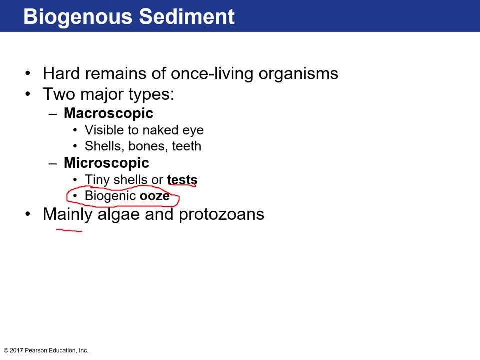 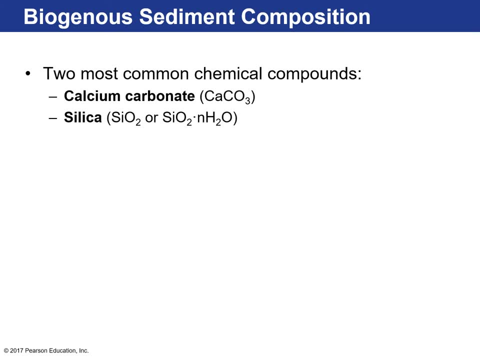 mud almost- and this stuff is made up mainly by algae and protozoans floating around on the ocean surface, so that's kind of the reason why it's called the surface. so the two most common chemical compounds that make up the biogenic sediment are calcium carbonate- okay, what kind of like the material that a lot of. 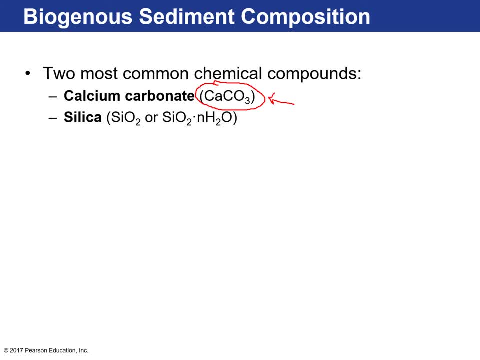 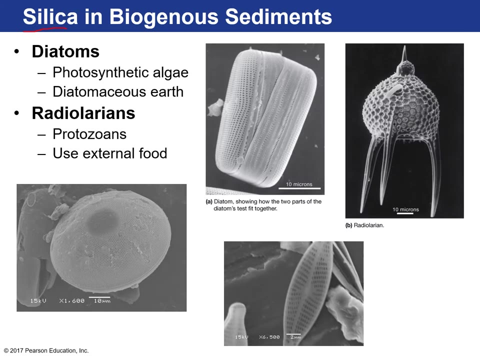 shells are made of that you see washed up on the beach, or coral, and then silica. okay, those are the two most common types of biogenic sediment, or they're the composition of biogenic sediment. so let's talk about the silica sediment first. this is mainly made up by these two different types of organisms: diatoms. 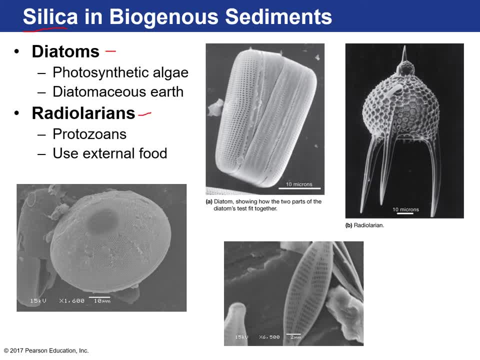 and red Euler. Ian's diatoms are single-celled, you eukaryotic, planktonic, photosynthetic algae, and they float around the surface of the ocean and they photosynthesize, so that's how they generate their food. this here, this image here and this image here, our diatom. 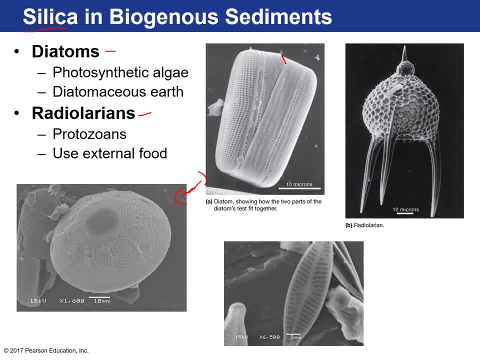 and they generally create these shells out of silica. You can see they're very beautiful and ornate. A lot of times diatoms, or almost all the time they have. you can kind of it's almost like a shoebox, where there's a top and a bottom and they close together. 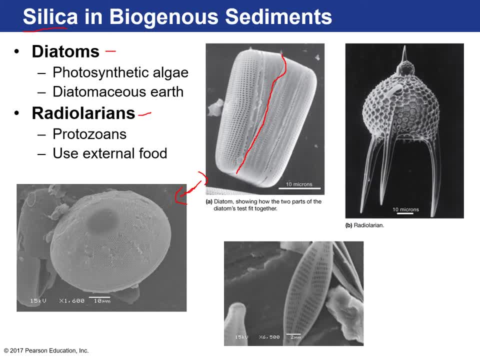 So they have two kind of symmetrical sides And the organism is a single-celled algae that lives inside this. These little holes that you see here are holes in the silica to allow nutrients in and waste to come out, And since they photosynthesize, that waste is oxygen. 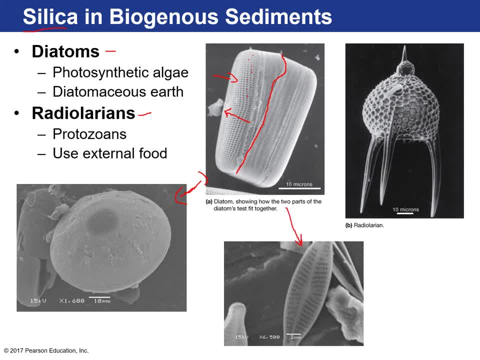 So, oh, down here, this is also a diatom as well, almost like a canoe-shaped diatom. down here And this one's more round, There are over like 7,000 different species of diatoms, So incredibly diverse, numerous in the ocean. 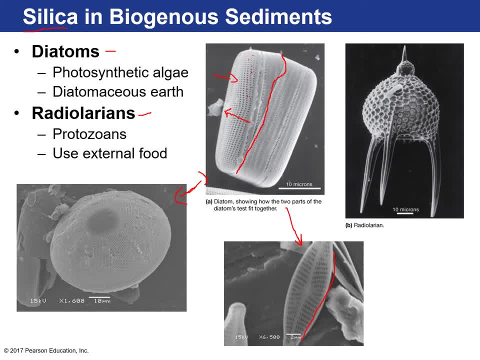 It's almost like they're the kind of grass of the ocean. They're small organisms that are just all over the place, photosynthesizing in the sunlit layers of the upper ocean. Okay, And then there are radiolarians. Radiolarians are protozoans. 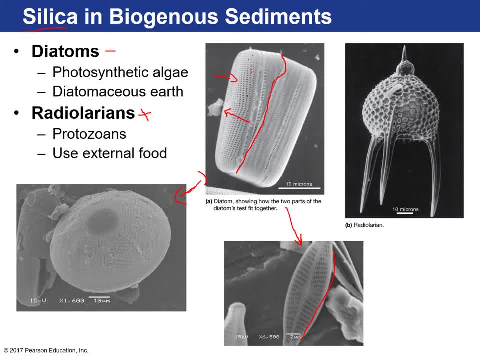 Most are planktonic, so they float around in the ocean, But they use an external food source. They have to kind of bump into other planktonic organisms to eat them. Okay, This right here is a radiolarian. Sometimes they're referred to as the snowflakes of the ocean. 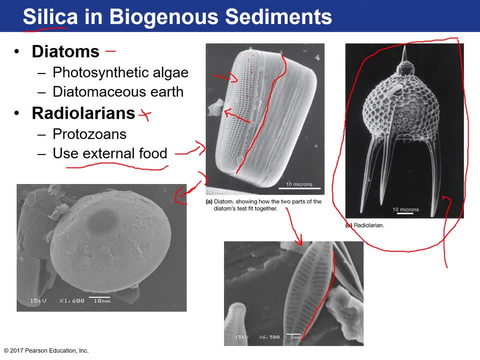 because of their beautiful and ornate creations. Okay, So again, single-celled organism, And they often have kind of these spines that shoot out of them And that's to help them float because they're planktonic. Okay. 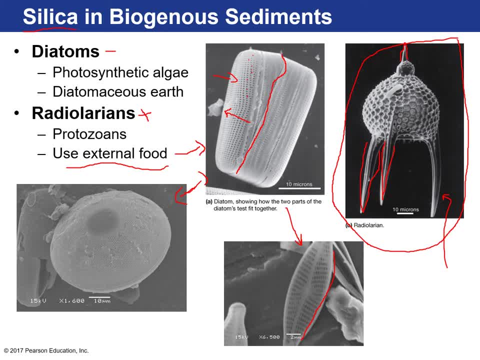 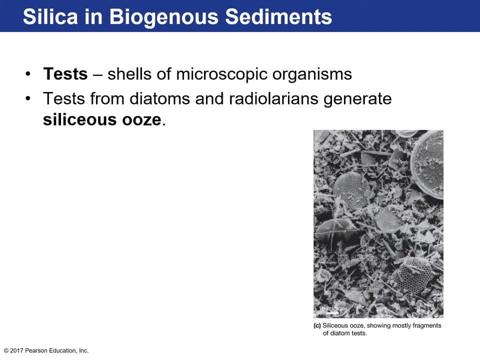 Very beautiful. They make all these tests or shells out of silica And when these organisms live and then they die, their shells rain down to the bottom of the ocean floor and that creates something called diatomaceous earth. Okay, It's kind of like this white powdery material that we actually use. 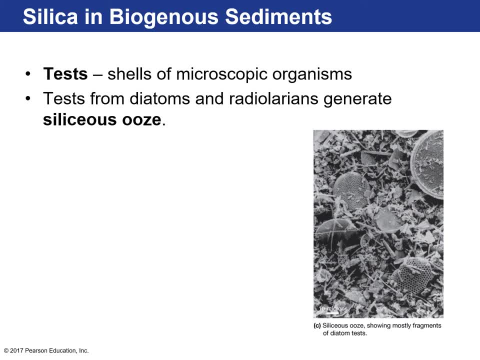 in a lot of different Household products at the time. So those are the tests. These are the shells of microscopic organisms. This is what broken down ocean sediment would look like under a microscope. If you have a lot of biogenous sediment in it, you can see some of the shells of diatoms. 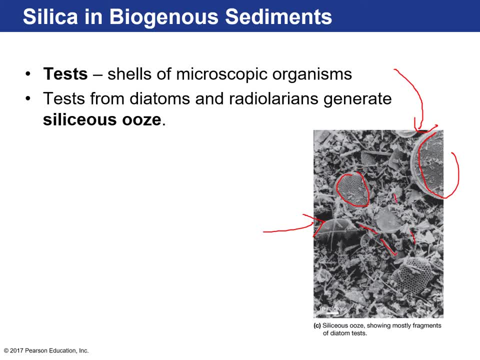 broken pieces of radiolarian all over the place, And that's what makes up siliceous ooze. So it's a biogenic ooze that's mainly composed of silica. Okay Now, siliceous ooze, in terms of sediment, it's defined as having: 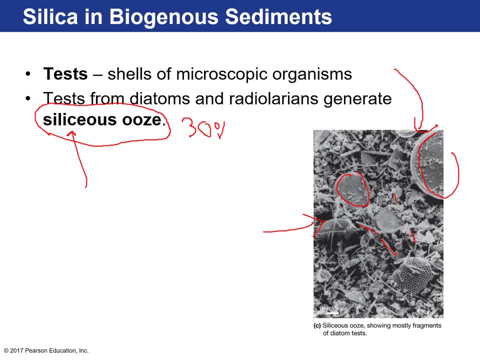 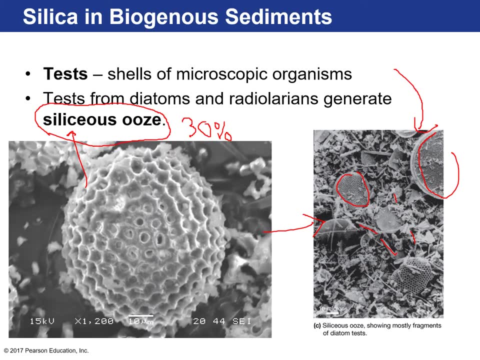 at least 30% ooze that comes from silica. The rest is typically very fine lithogenous sediment like clay, but it's still considered an ooze. Oh, so here's another radiolarian. We, actually one of our oceanography classes- took this image using a scanning electron microscope. 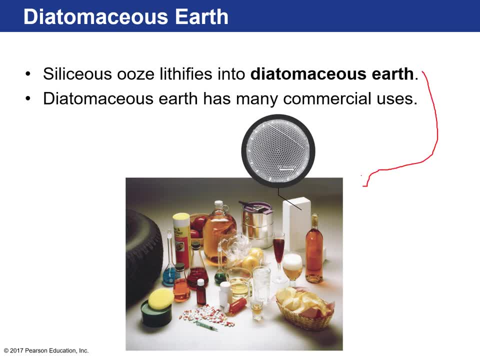 So diatomaceous earth, like I mentioned, has a lot of sediment. It has a lot of uses. We use it as a water filter, We use it in the production of beer- yay, bread, cleaning solutions, fillers and tires. 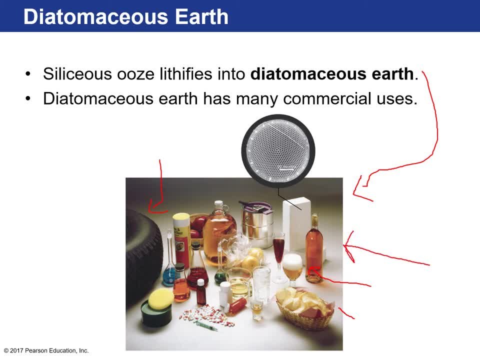 And, kind of oddly enough, we use it as an abrasive. It's put in toothpaste, So when you brush your teeth the silica is a very strong mineral so it could polish your teeth, So that's why We use it in that fashion. 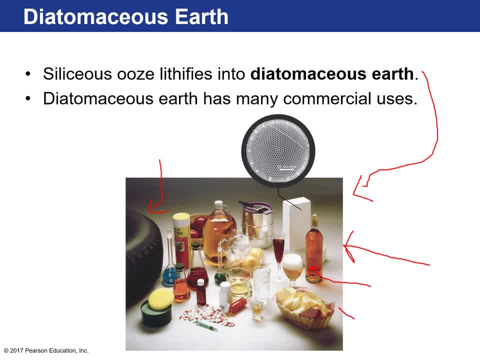 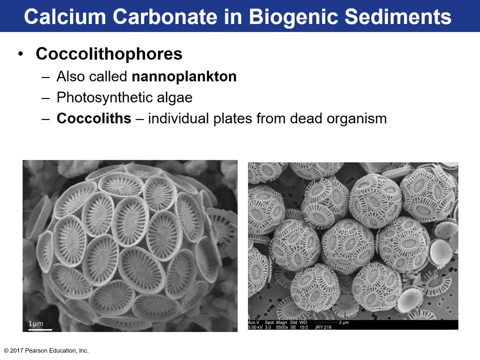 So perhaps this morning you brushed your teeth. Little did you know you had these, the dead remains of microscopic marine organisms, just their bodies used to scrub clean the teeth in your mouth, really Okay. then there are the calcareous oozes, or the calcium carbonate biogenic sediment. 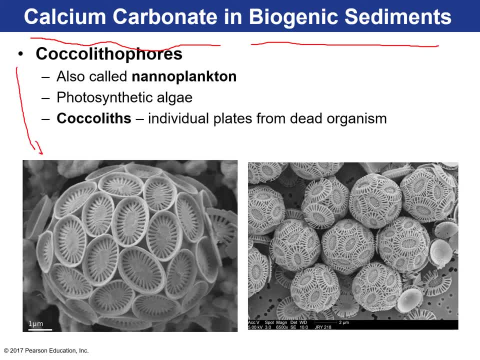 Okay, these organisms are much smaller than diatoms. These are coccolithophores, and what they do is they create these plates and they surround themselves by these plates, which eventually make a circle, But they also- these are photosynthetic algae as well, so they photosynthesize as well. 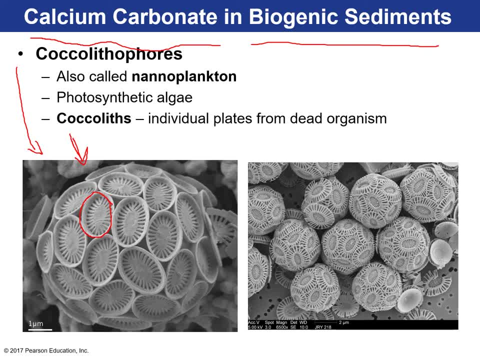 They're just much smaller. A lot of times they're called nanoplankton because they're much smaller than diatoms. By the way, diatoms are found almost in every environment. They're found in like ocean sediment, you know. they're found floating in the surface. 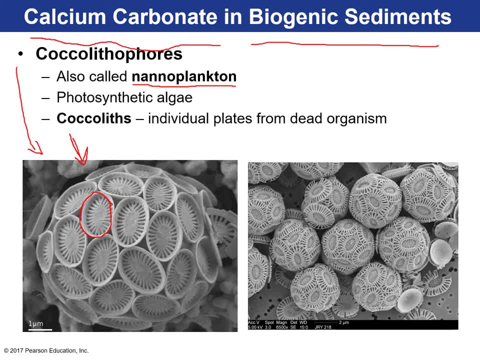 of the ocean, kind of by themselves or in communities. They also live on the skin of sea turtles and also whales, So you find these organisms all over the place. So when coccoliths die, then their tests, which are made up of something different, 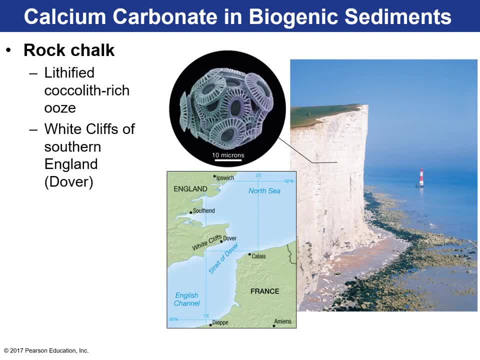 calcium carbonate also sink to the bottom of the ocean And if enough of this accumulates to form calcareous oozes and if that lithifies to form a rock, that's where we get rock chalk from. okay, These are the White Cliffs of Dover. 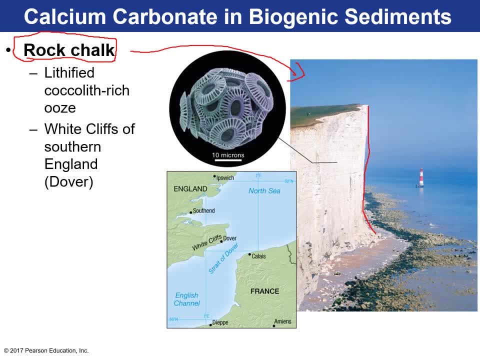 This is an entire cliff made up of chalk, Like so you could go over here and chisel out a piece of chalk and then just start writing on a blackboard, And that's pretty crazy. Think about that, right? So this material, which we use often when we teach in person- and we'll get back to that- 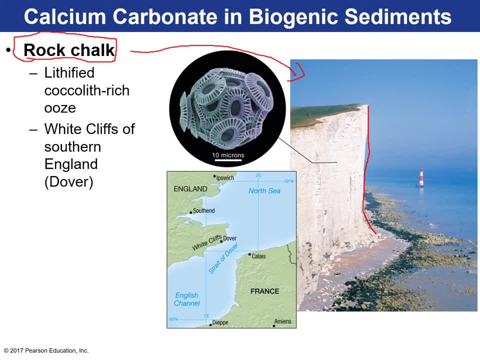 but you're essentially just smearing the lithified remains of dead marine organisms as you're trying to explain some sort of complex calculus theory or physics problem which is kind of intense, all right. So here's: the best example of this are the White Cliffs of Dover. 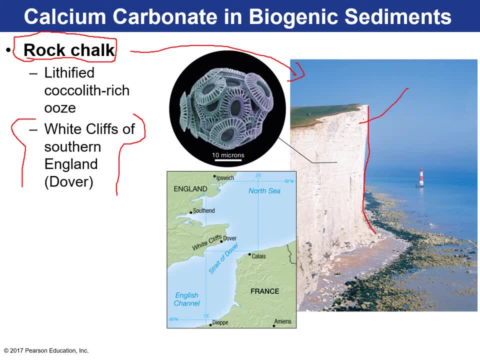 There are a lot of these White Cliffs age to the Cretaceous time. In fact, there are a lot of different chalk deposits around the world on land that date back to the Cretaceous. The Cretaceous is kind of a. it's named the Cretaceous because there are a lot 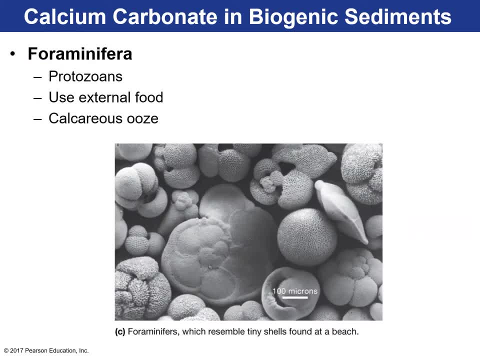 of chalk deposits. as a result, Foraminifera, another type of organism, protozoan, that also needs an external food supply. They also become part of the calcareous ooze when they die and become part of ocean sediment. These are much larger than coccoliths. 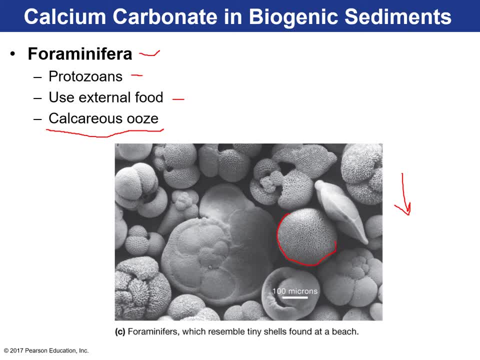 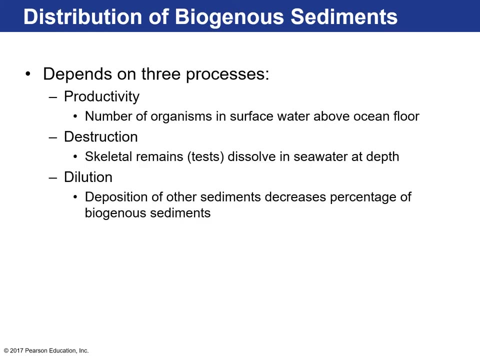 A lot of times they're buried in the sediment. Sometimes they can float around in the water, It just depends. There's a lot of different species, but yeah, they're made up of calcium carbonate. Okay, so the distribution of biogenous sediment really depends on three things. 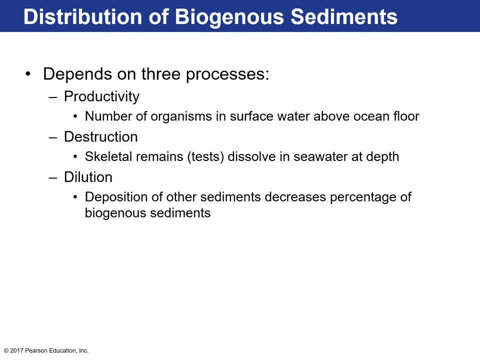 The productivity, meaning the number of organisms in the surface of the water above the ocean floor. So if you have a big bloom of these organisms and they're being very productive and reproducing and there's a lot of them, that means that you'll probably find a lot. 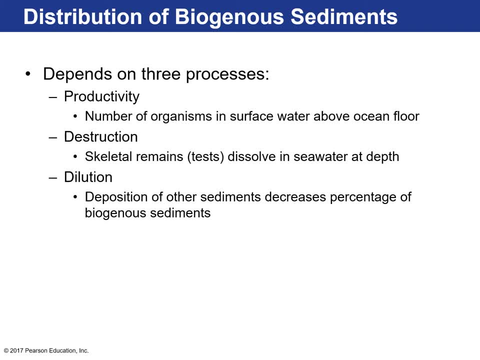 of biogenous sediment. You'll find a lot of biogenous sediment directly beneath them. Another factor is destruction, meaning that those skeletal remains or tests they can dissolve in seawater, especially at different depths, under different conditions. So if they're all dissolving away, then they won't deposit and you lose that material. 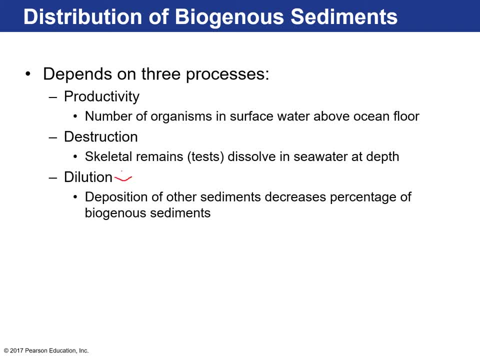 And the final factor is dilution, because in reality, most marine sediment is lithogenous sediment. So if you're in an environment that's very close to land, there are microscopic marine organisms that live in the surface waters there, But because so much lithogenous sediment is being delivered to the ocean in that area, 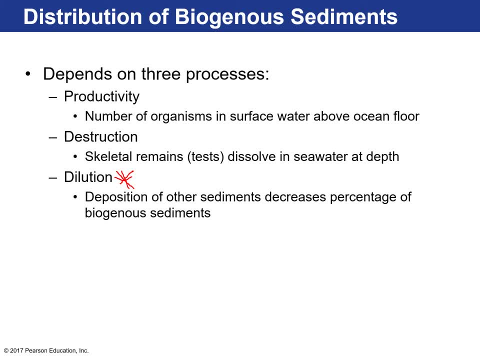 it dilutes the amount of biogenous sediment. So you'll find biogenous sediment in neuritic environments, but it won't ever be classified as a biogenic ooze just because there's so much more lithogenous sediment. So that's what dilution really is. 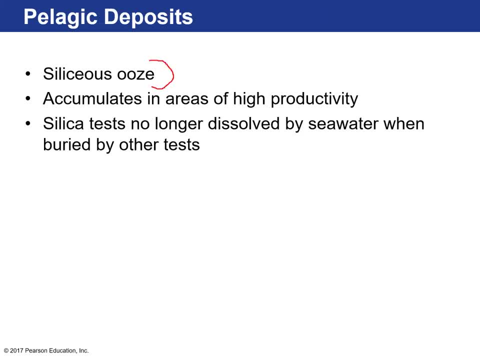 Okay, so let's talk about the biogenic ooze. Okay, so let's talk about the biogenic ooze. Okay so let's talk about the biogenic ooze. Let's talk about siliceous oozes. They accumulate in areas where there is really high productivity. 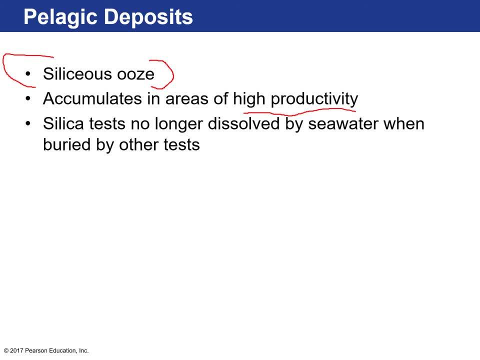 meaning that these organisms are proliferating, ubiquitous, all over the surface of the water. So silica tests do dissolve in ocean water, but they do not dissolve if enough is being produced and varying the ones that hit the bottom of the ocean. So let me show you an image of what that looks like. 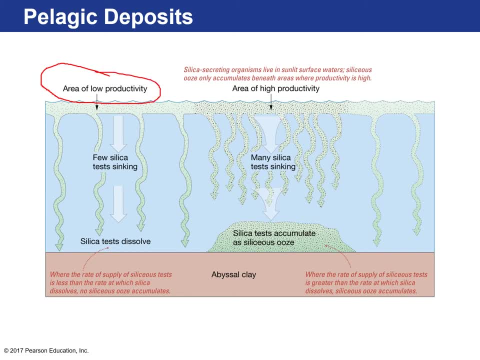 Okay, so say we have an area of low productivity. Not too many organisms are living and dying that create those shells, so very few tests are sinking. And because very few of them are sinking, they're all dissolving either before or when they get to the ocean floor. 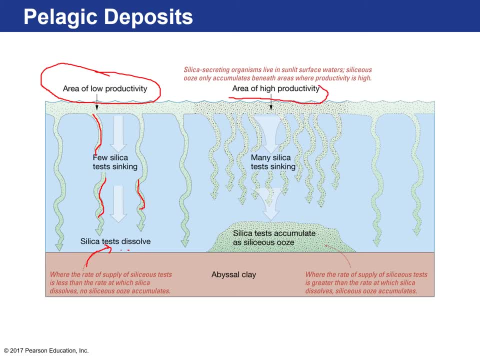 Okay, but if you have an area of really high productivity, then that means so many shells are coming down and depositing out so quickly that there isn't enough time for them to dissolve away. So a lot of these siliceous oozes are not dissolving. 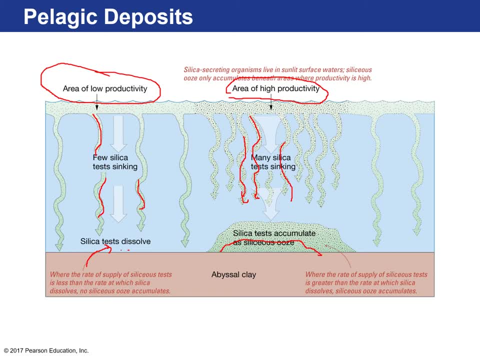 Okay, so let's talk about the biogenic ooze. siliceous tests are preserved essentially by burying more and more silica tests above it, And this is how you would get a siliceous ooze deposit. So they really occur in areas of really 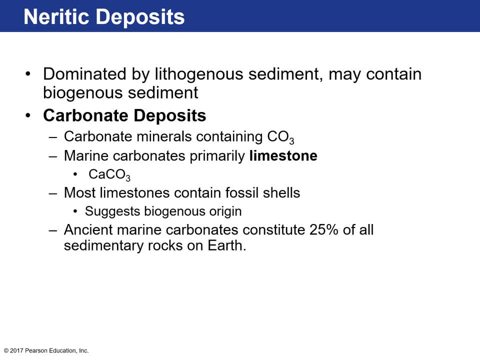 high productivity. Now, neuritic deposits are, like I said, dominated by terigenous or lithogenous sediment. They can contain biogenous sediment, but again, it's the dilution thing. You don't really find, or you can't find them in really high concentrations because there's just so much. 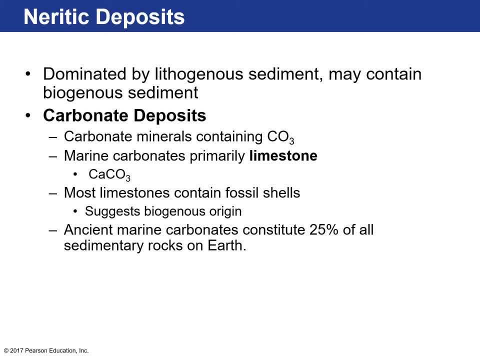 lithogenous sediment. Carbonate deposits are deposits that have a lot of CO3, okay, carbonate minerals that contain that in it. Marine carbonates are primarily limestone, which is calcium carbonate, CaCO3.. Most limestones contain the remains of living organisms. 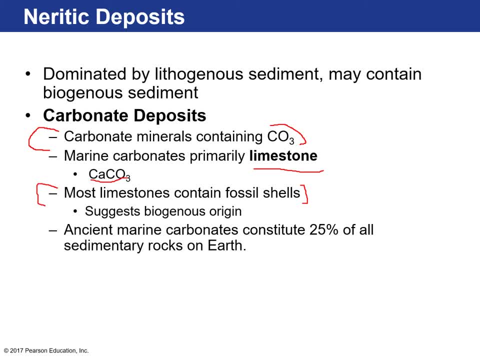 You can find them in the environment, but they're not really found in the environment. You can find, like coral or other bivalves or shells, And so that really suggests a biogenous in origin, And so a lot of the ancient marine carbonates make up about 25% of all sedimentary. 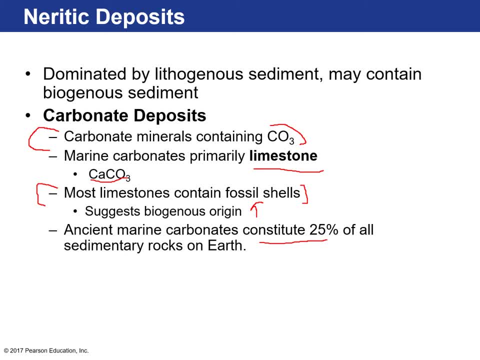 rocks on Earth. We have a lot, In fact. the top of Mount Everest, the rocks that you walk on as you're at the highest point on Earth, are limestones. Those have an origin In the ocean. in shallow oceans There's huge deposits of limestone. I mean Florida, the entire. 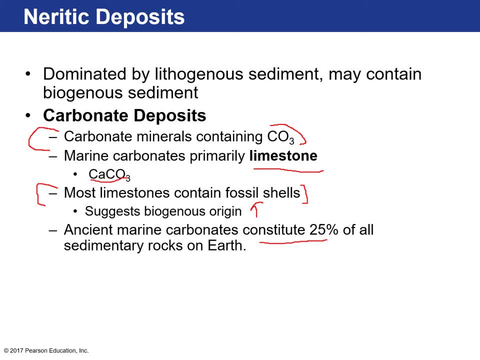 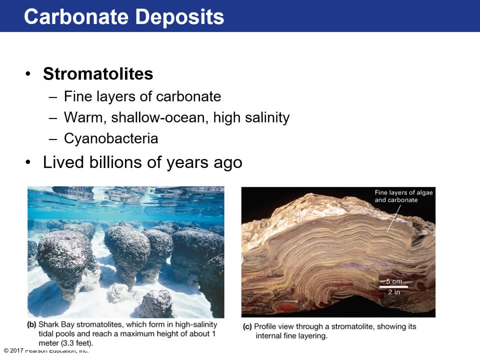 state of Florida, our bedrock is all limestone. Parts of Kentucky are kind of like that. Places in Central America have a lot of limestone, like the Yucatan, So there are a lot of places that have limestone as their bedrock and that's kind of derived from ocean environments- Stromatolites. 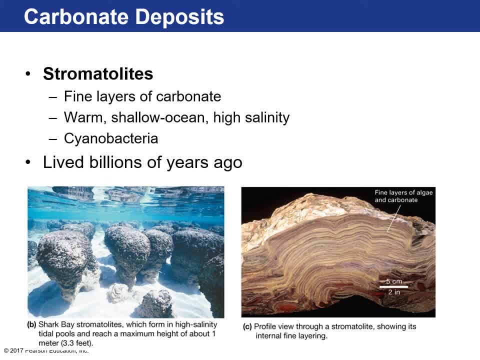 are an organism that is a type of limestone. They're a type of limestone that is a type of limestone. They're a type of carbonate deposit: Stromatolites. they still exist today in Sharks Bay, Australia, but they lived billions of years ago. Some of the oldest evidence of life we have on 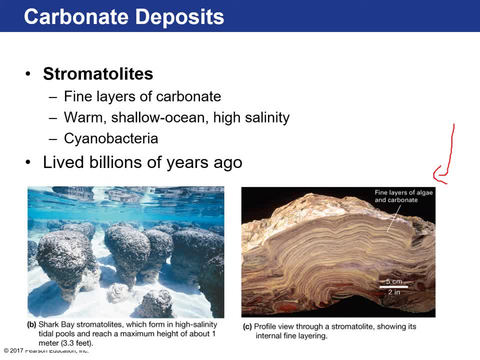 Earth are from stromatolites And the way they live is they kind of create this bacterial mat and accumulate sediment and then they just kind of build on top of it. So there's these concentric layers of a colony of bacteria, photosynthetic bacteria, that just kind of grow one on top of. 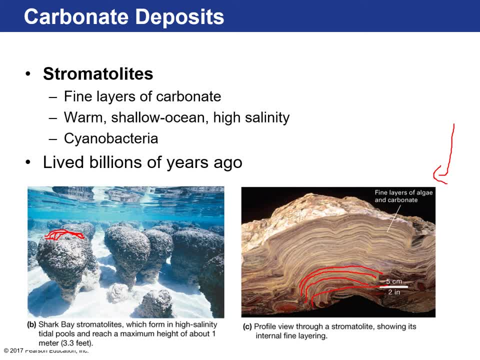 each other, And so you can see the fine layer of carbonate, different kind of almost like growth rings in a tree. Stromatolites are a type of cyanobacteria and they kind of this only forms in very warm shallow seas of high salinity And they're still around In Shark Bay, you can see. 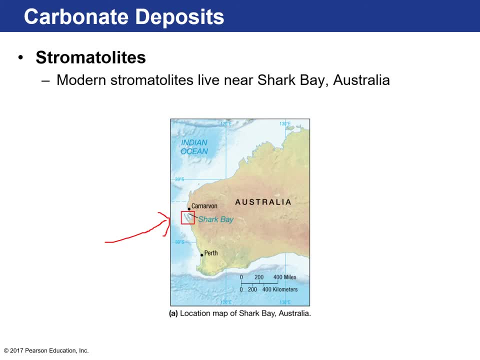 modern stromatolites. They existed 3.5 billion years ago and they were really the first evidence of photosynthetic life. And they're still on Earth And a lot of times they're attributed to oxygenating our atmosphere. 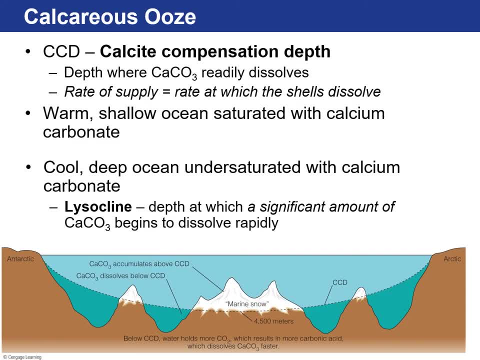 so they were really important that long ago. But a lot of carbonate material, especially out in the open ocean, deeper parts of the ocean, dissolves away. The calcareous ooze only forms in kind of shallow portions of the ocean floor, And the reason is because calcium carbonate readily dissolves. 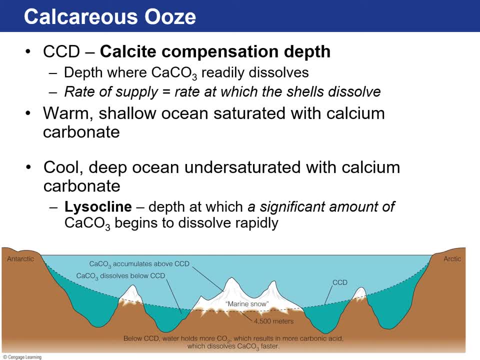 especially when the temperature drops and ocean acidity increases. Those are kind of the two factors that are most important. Calcium carbonate is a very strange material because it precipitates out in warmer waters, So like I don't know if you've taken a warm shower, but a lot of times 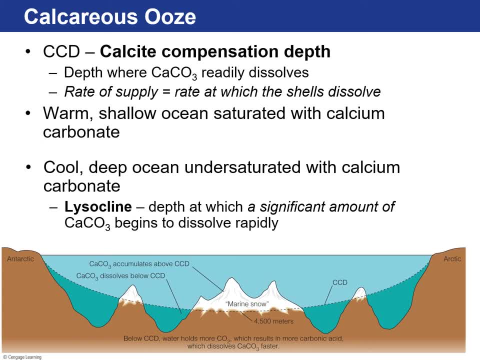 you see, like this white crusty stuff form on your showerhead. That's calcium carbonate, because you're like, oh, that's a lot of calcium And it precipitates directly out of the water- our Florida water- because it has a lot of calcium in it. So it'll precipitate directly out of the water onto your showerhead. 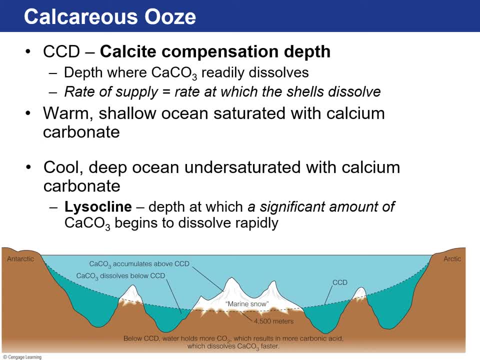 So yeah, so we see this in the ocean, But in the ocean, especially in the deep ocean- see this area down here- It's very cold. So when it gets very cold and when there's a lot of carbon dioxide in the water itself, 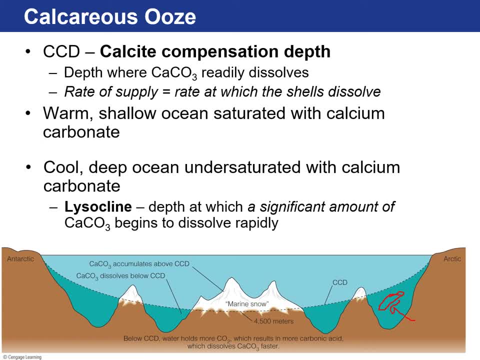 that raises the acidity of the ocean. So it's very cold And it's very hot And it's very cold And it's very cold. You can tell if you're in the ocean by adding some calcium carbonate. it will help with the acidity of the water. 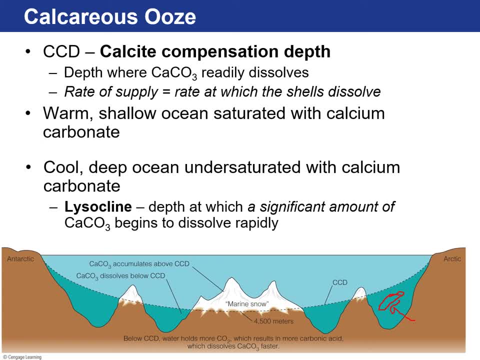 And then helps dissolve away a lot of the calcium carbonate. Okay, so what happens is there's a depth where calcium carbonate readily completely dissolves, And we call that the CCD, the calcite compensation depth. So here the rate of supply equals the rate at which the shells dissolve, And then none of this material will. 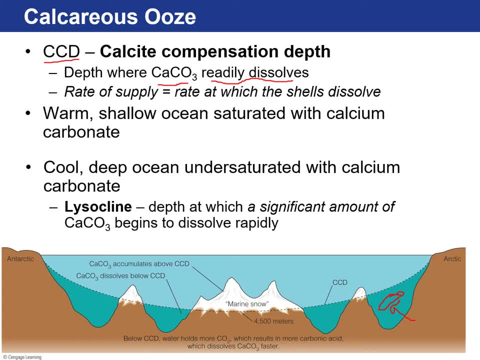 deposit on the ocean floor. So really a lot of calcareous oozes will form in more or less all over the ocean, And this is really a big difference. We'll walk through some more detailed examples of these with you. shallow areas of the ocean: okay, when you have cool deep ocean that's saturated in calcium carbonate. 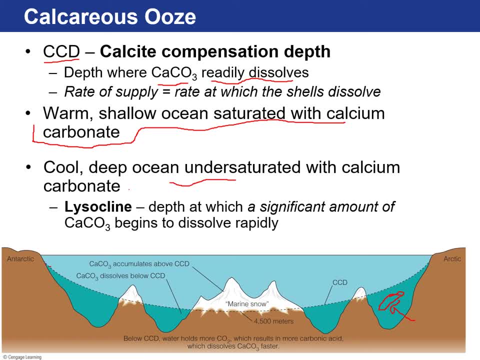 then you'll have a ccd. so this dashed line here is the carb, the calcite compensation depth. so if you have any organisms that live on the surface of the ocean, here, their material, their tests and shells will rain down and then, as they hit this limit, which is typically on average, 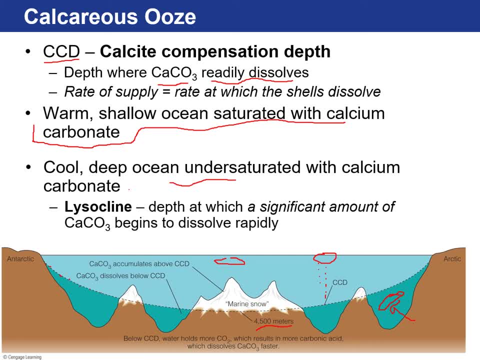 four and a half kilometers beneath the ocean surface. they'll readily dissolve away and you won't find any calcareous oozes beyond this depth. but there are places of the ocean floor that are at a higher- quote-unquote- elevation, let's say- and they're above the ccd, and so they'll deposit in. 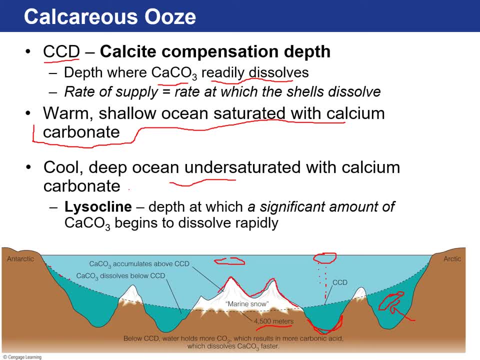 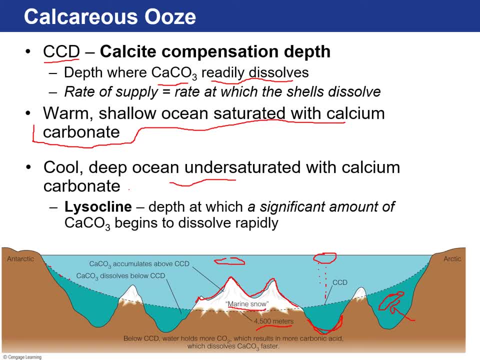 it's like marine snow, so you can think of calcium carbonate from these microscopic organisms falling down and depositing in high areas of the ocean floor above the ccd. okay, and the reason why it's below the ccd: the water, because of that higher pressure, can hold more dissolved carbon dioxide. 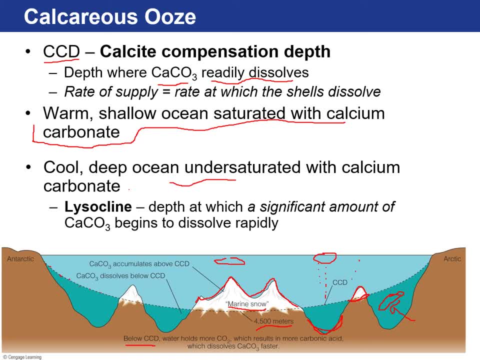 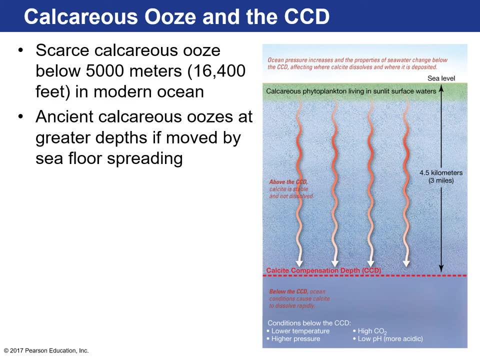 and if it holds more carb carbon dioxide, that creates more carbonic acid, which makes the water more acidic, and that's why calcium carbonate dissolves faster beyond the ccd. so you really find- you don't find any calcareous oozes depositing beyond about five kilometers. 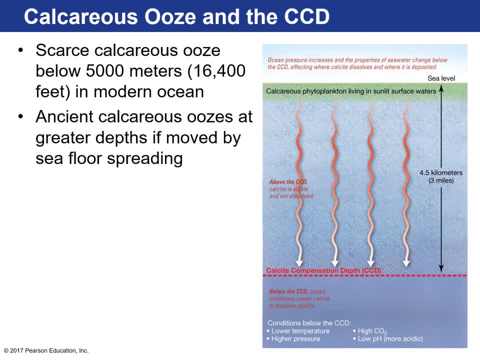 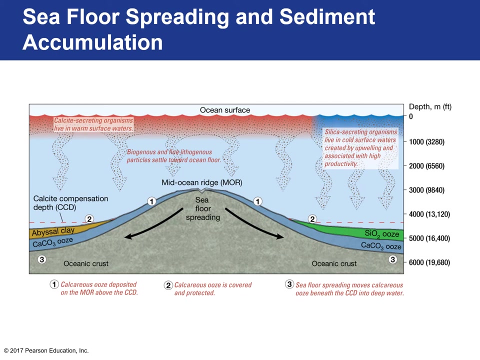 okay, in our modern ocean, ancient calcareous oozes may have deposited a greater depth, depending on different situations in ocean chemistry. also, uh by plate, tectonic situations like, uh, seafloor spreading. let me show you an example of that. so the mid-ocean ridge: okay, this is where we have active volcanism and new ocean plates being. 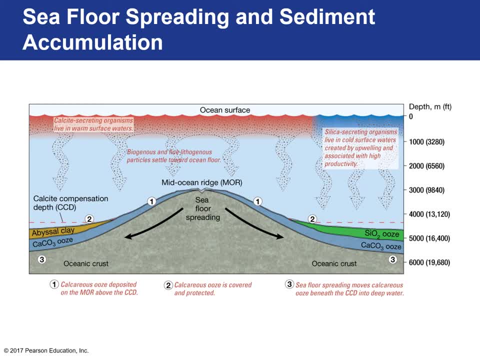 created. this is at a higher elevation than the average ocean floor and the reason is because it's hot and it's more buoyant. you have new ocean crust rising up and you have volcanic eruptions right at the center of the mid-ocean ridge. so, on the ocean surface, biogenesis. 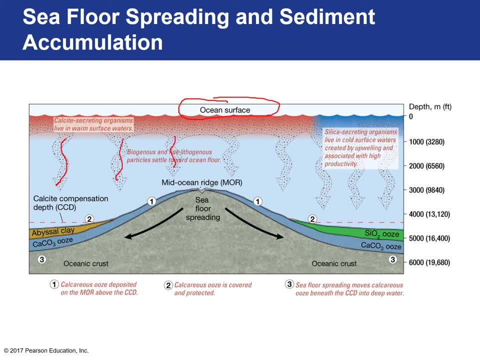 sediment is being produced and it's raining down on the ocean floor, but over here all that vaginous sediment is depositing below the ccd, so it just dissolves away over the mid-ocean ridge area, which is like here. this entire environment is above the ccd, so what you'll find is see this blue. 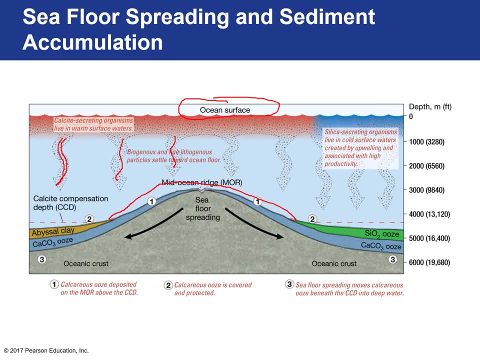 kind of wedge here. that blue wedge is calcium, uh calcareous ooze, depositing on the mid-ocean ridge. but over time, as the two plates diverge from each other and they move away from the mid-ocean ridge, the plate kind of moves downwards into deeper waters. but what happens is: 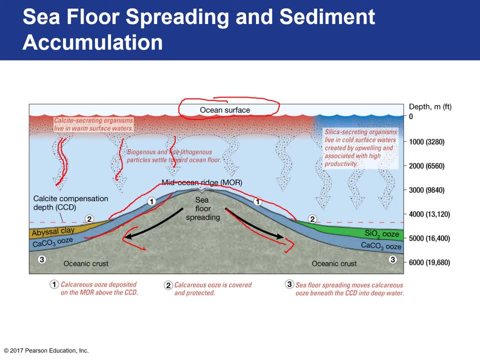 so much abyssal clay has been depositing on top of the calcareous ooze that the calcareous ooze actually gets preserved underneath the abyssal clay and, despite the fact that it's below the ccd, it has a protective layer above it so it doesn't dissolve away. 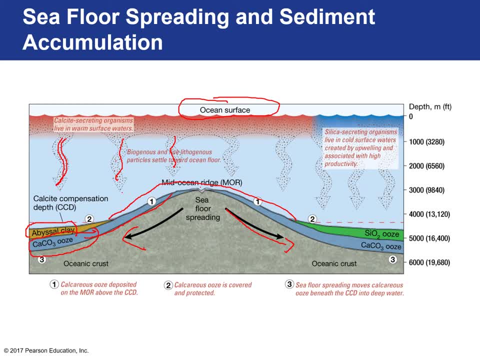 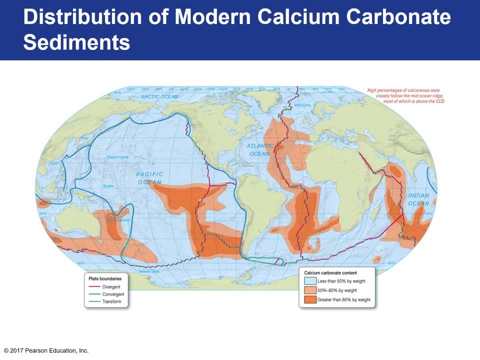 so that's a a way that seafloor spreading can affect sediment accumulation. so here's the the modern distribution of calcium carbonate sediments. uh, in our oceans, if you notice, they kind of um are depositing in the more shallow areas of the deep ocean, closer to mid-ocean ridges. you see how, see how they're kind of. 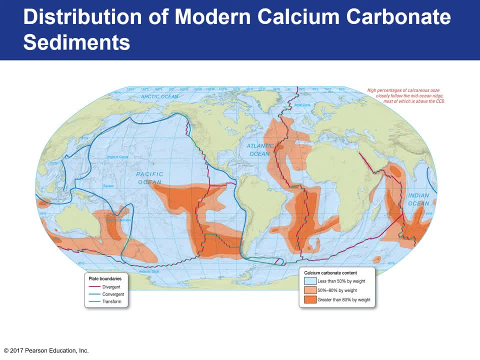 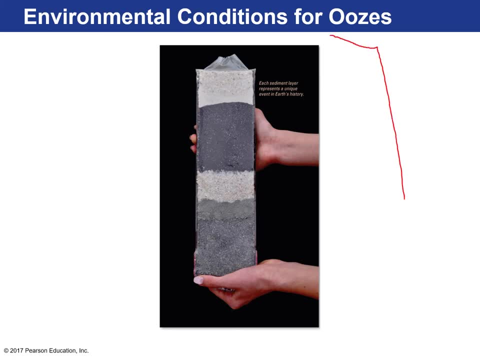 all over the mid-ocean ridges, and that's because typically those areas are above the ccd, all right. and then here are another example of a cross-section of marine sediment. so perhaps you know, um, the changes that you see here in coloration might be changes uh of um, as the 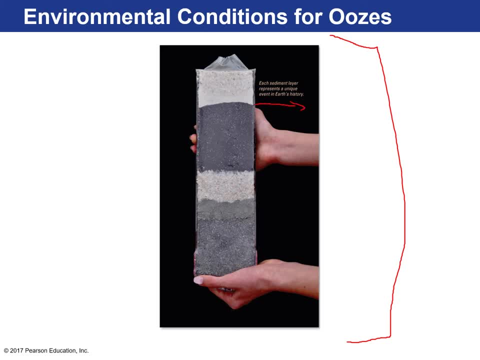 ocean floor is moving away from the mid-ocean ridge, then you get deposits of of abyssal clay above what would be biogenesis and that that would be preserved. so that's what can account for these major changes in marine sediment over time. all right, let's talk about hydrogenous marine sediments. these are ones that 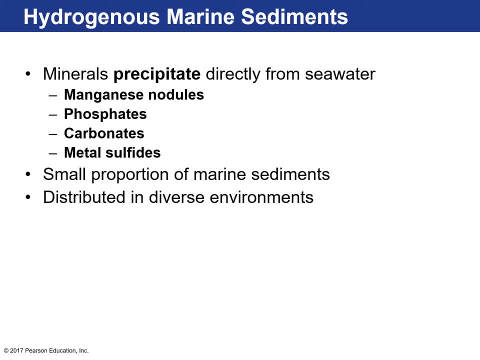 precipitate directly from seawater. okay, and there are many types think of. what i mean by this is think of like, say, you have water, right, and you add a bunch of sugar to it, okay, and then you heat up that sugar. that sugar will crystallize into something. it's basically a little bit of a residue of water that, if it gets. 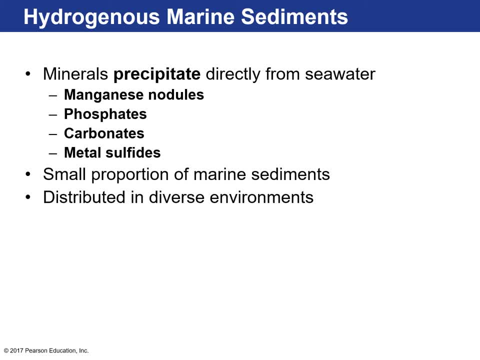 separated from a sieve, it will start to precipitate out and eventually, if the temperature goes up high enough and there's a little bit of evaporation, the sugar will saturate in the water and then begin to precipitate out. that's what hydrogenous marine sediments are: different materials dissolved. 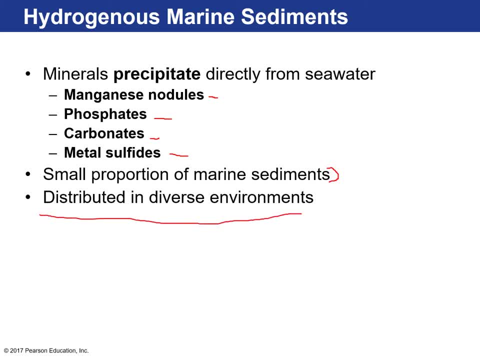 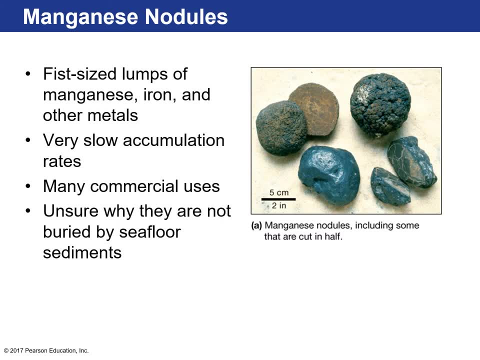 in ocean water that precipitate out and then deposit on the ocean floor in a very diverse types of marine provinces. Okay, let's talk about manganese nodules first, because they're really the most interesting. They're almost like golf ball sized pieces of mainly of metal, mainly manganese. So what's that doing at the bottom of the ocean? It's crazy. 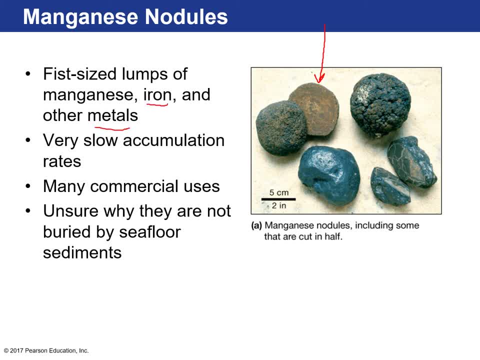 They have a lot of iron in them. other metals- copper. They grow very slowly, Their accumulation rates are very slow and they have a lot of potential commercial uses. So people have thought of mining these nodules that are found on the surface of the deep ocean, which is very weird. 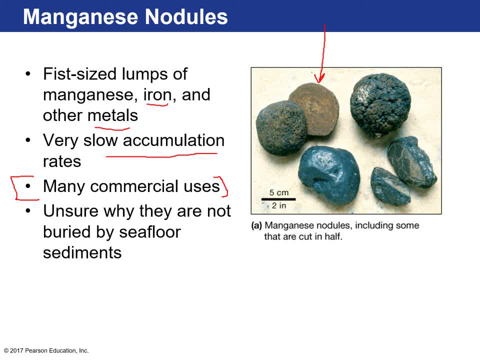 Scientists still aren't unsure exactly how they form. They know that if you cut them open you typically find like a shark tooth or a piece of fish bone or perhaps a lithogenous sediment and the metal grows around it. They think there's some sort of bacteria that slowly accumulates the manganese surrounding some. 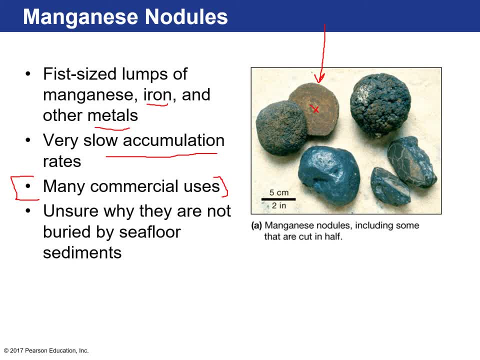 sort of nucleation piece, But they're really unsure why they're not. they take so long to grow, why they're not buried underneath all the other pelagic sediment out in the deep ocean. So something is kind of keeping it up on the surface. So, if you look, here's an image of the 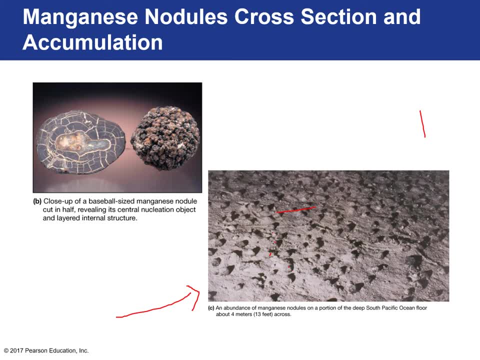 bottom of the ocean floor. You see all these manganese nodules just littered everywhere, And the density of them on the ocean floor varies on location. Some of them you have really dense areas and some, I guess, a little more sparse. But here's a cross-section of one about a baseball. 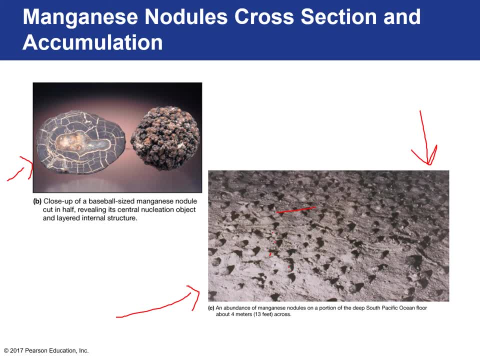 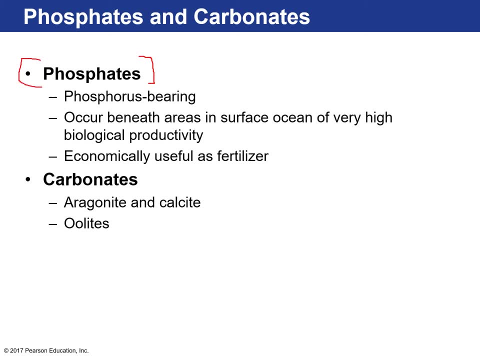 size manganese nodule- Okay. Phosphates: These are phosphorus bearing deposits. They typically occur in areas where there's a lot of biological productivity- Okay, Meaning that, like there's a lot of ocean life. Maybe this is a site of upwelling where nutrients went up to the surface. You get algal. 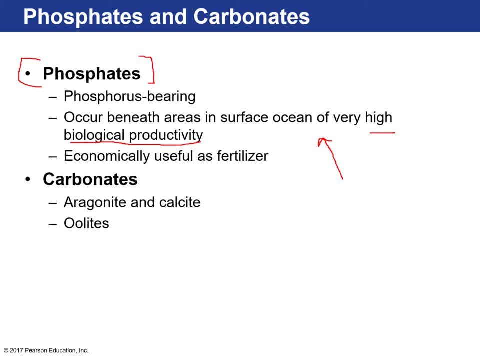 blooms, that brings in small fish and birds and then whales and stuff like that. So an area with a lot of biological productivity, a lot of organisms dying and that material kind of sinks to the bottom of the ocean floor there. And these, these deposits are very important because we use 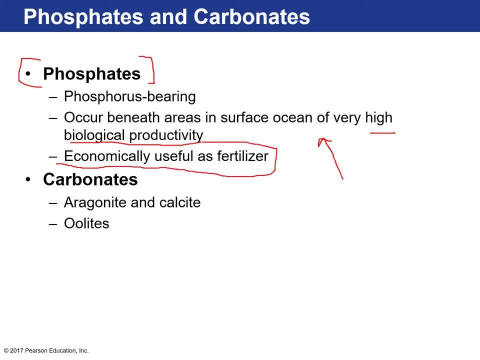 them as fertilizer. We actually have some, a lot of phosphate deposits near the Tampa area here in Florida. And then there are carbonates. Aragonite and calcite are the different types of carbonate deposits. Oolites are a type of carbonate that forms in very warm waters. It's calcium carbonate just. 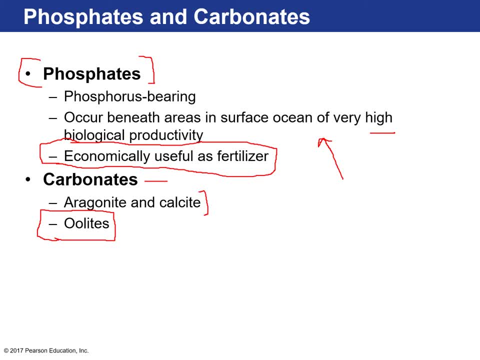 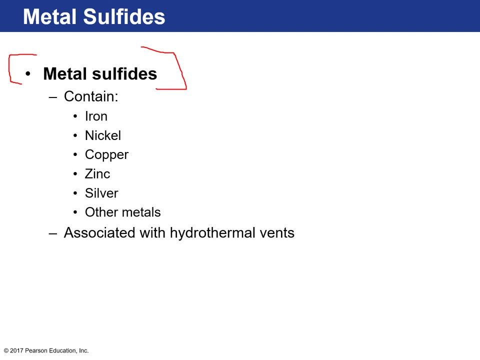 precipitating out of small circular nodules that roll around in the kind of waves in tropical areas. Then there are metal sulfides. Metal sulfides are made up of iron, nickel, copper, zinc, silver, other precious metals And they form from hydrothermal vents. 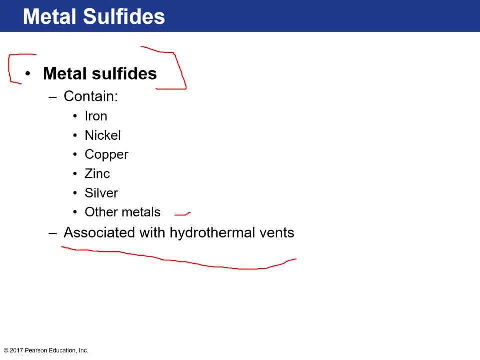 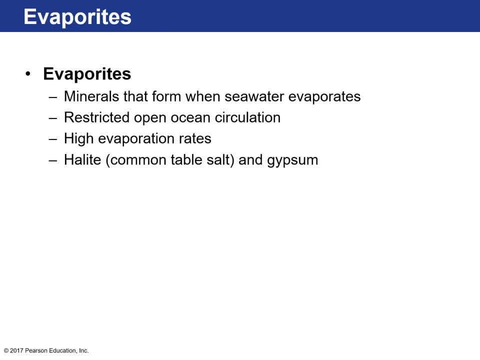 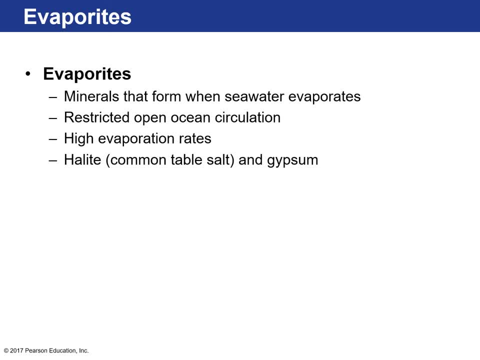 that form when seawater evaporates Comes from the name. This occurs in restricted, kind of cut off ocean areas with restricted ocean circulation, really hot and dry areas, high evaporation rates, And what will happen is as the, the ocean waves shift near your звучes, you will begin to see those 모 illness, with course to experience and 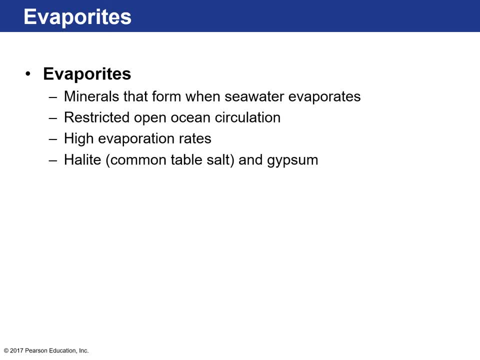 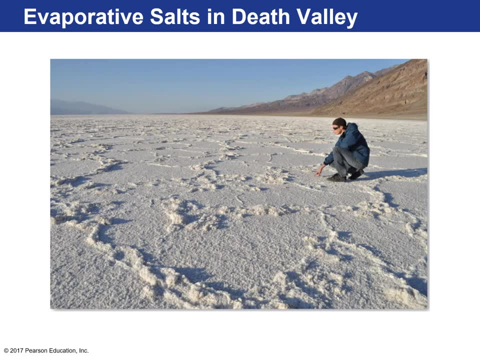 water evaporates, you'll start to precipitate out halite, which is table salt, and also gypsum. In fact, at the bottom of the Mediterranean Sea there are vast deposits of gypsum and halite, which indicates in the geologic past the Mediterranean Sea has completely dried out. 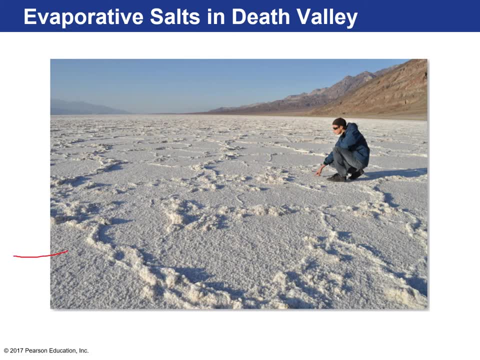 and left behind deposits. like you see here, This is a salt flat in Death Valley in California, and so here this is all: white gypsum and salt and halite over a vast area. This area is really dry, so anytime it rains, all this water kind of goes out into this low-lying valley and then 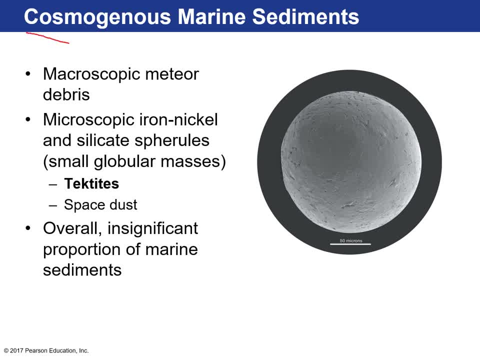 evaporates away. And then finally, the last type of sediment are cosmogenous marine sediment, and these are derived from meteor debris. okay, Microscopic iron and nickel, silica spherules can kind of come into our upper atmosphere. They get heated up and some of them melt. They turn. 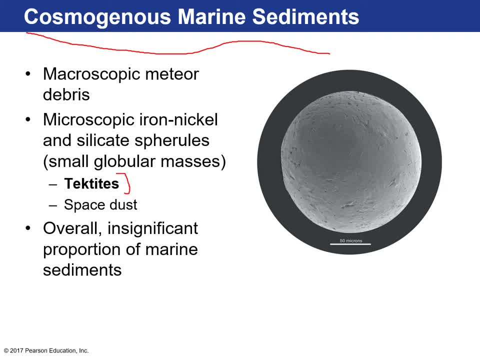 into tektites which are made of glass, and those can deposit out into the ocean floor. okay, They're really an insignificant proportion of marine sediment, I mean really small amount, but they can indicate major events, perhaps major collisional events that have occurred in Earth's. 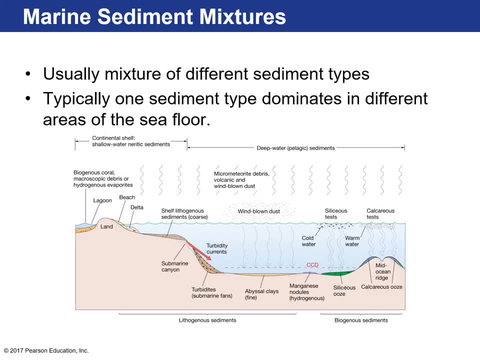 past. Okay, so here it is. This is the summit up kind of cross-section of the ocean floor, showing you like different parts of the ocean. Usually, when you go down and sample all the marine sediment, you usually find a mix of different types of sediment, all the different types of. 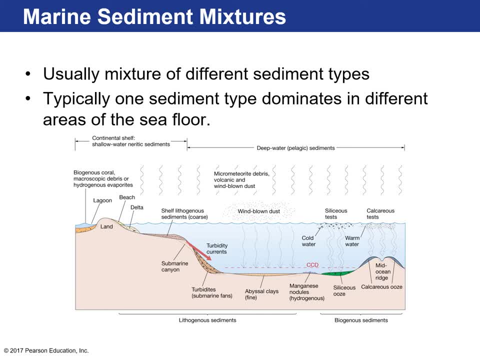 sediment we talked about before, okay. So, for example, if we're closer to land, okay. in lagoons we would find biogenous, coral, macroscopic debris or even hydrogenous, or even chemical, which would essere said to be like the elixir of earth. 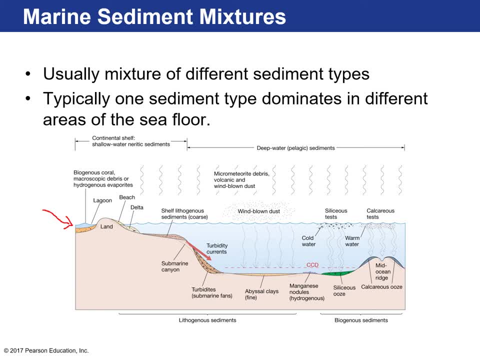 But what we did was: okay, compare this with the ocean floor, where there's more sediment. the ocean floor would have more sediment. We're going to dig deep into the ocean floor. so let's say: this is the ocean floor. right, That's the ocean floor of the ocean floor. 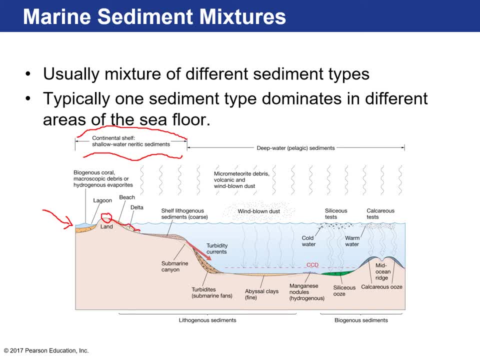 And this is the ocean floor of the ocean floor. right Here's the ocean floor where we find large amounts of sediment that evaporate the ocean floor and it evaporates kind of like land-locked areas, no ocean circulation. 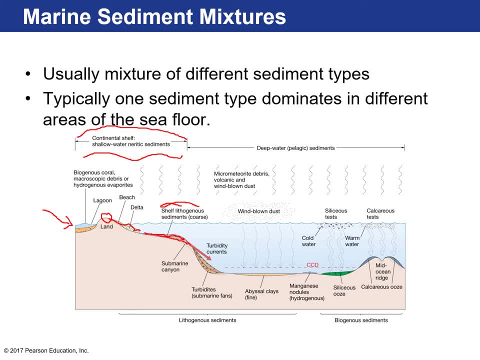 Here's land, here are beach deposits, here's the delta. okay, Here are those submarine canyons. and then turbidity- currents, under the force of gravity, bring a lot of sediment down towards the abyssal plains. So here are those turbidite deposits, or submarine fans. 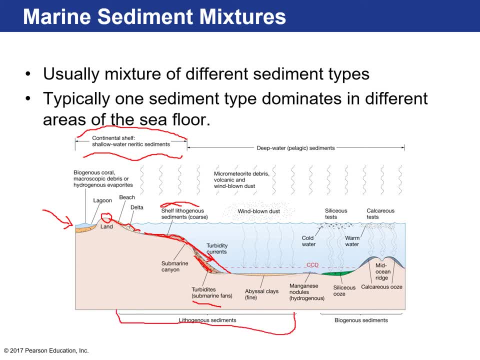 This is really the extent of lithogenous sediments that we would find, based on their origins on land. Wind-blown dust will make it out to these deep parts of the ocean and they'll slowly settle to the bottom and become abyssal clays, fine clays, mostly made up of lithogenous. 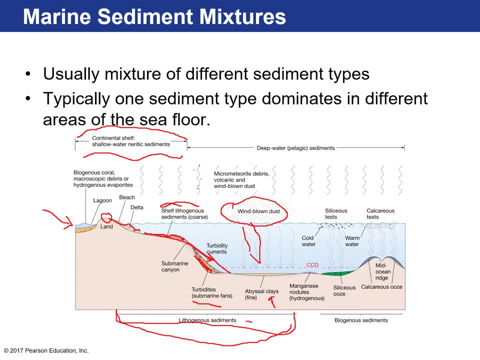 sediments. Remember all the while, microtactites and debris, volcanic wind-blown dust- can deposit in any of these environments, So there'll be a small amount in those in pelagic sediments. So once you go beyond the continental shelf, then you're into the deepwater pelagic sediments. 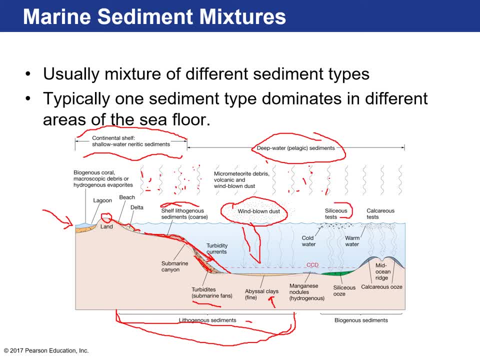 In deepwater pelagic sediments, you'll start to see microscopic organisms depositing sediment. These are called salacious tests or calcareous tests. Calcareous tests will not dissolve at higher elevations in the ocean above the CCD, So you'll see deposits of calcareous oozes in places like mid-ocean ridges. 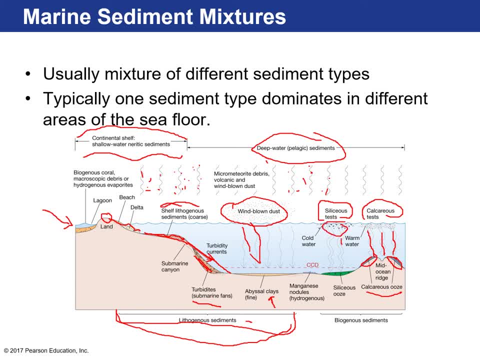 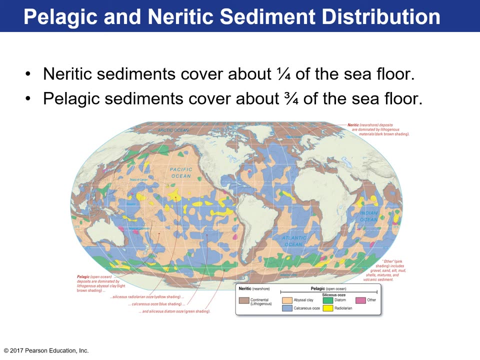 Then, in deeper parts of the ocean, where there's high productivity, you will see deposits of salacious oozes and that rounds up your biogenous sediments- Boom, Okay. So how is it distributed? Well, in terms of coverage of the ocean floor, neuritic sediments only cover about one-fourth. 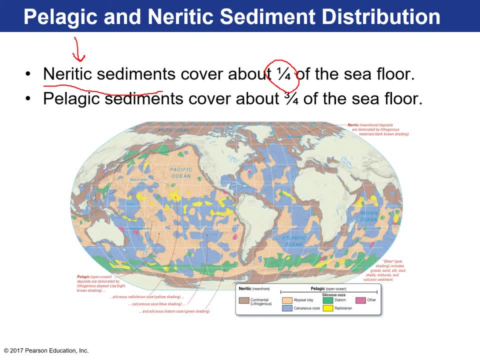 of the sea floor, meaning that the sediments that are close to land only cover about one-fourth of the sea floor. That makes sense because there's a lot more open ocean than there is ocean surrounding land. Okay, So pelagic sediments, in terms of coverage of the ocean floor, cover about 75% of the 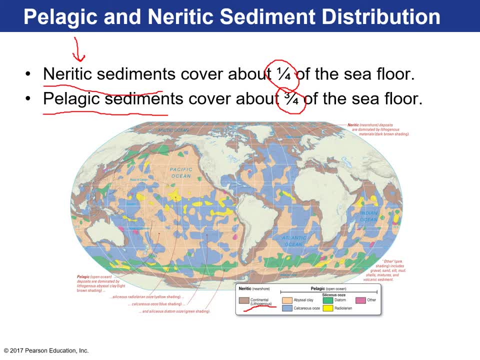 ocean floor. Here you can see, based on the different colors, the different types of sediment: abyssal, clay, calcareous oozes, diatoms, radiolarian, breaking down some of those pelagic sediments on the open ocean. 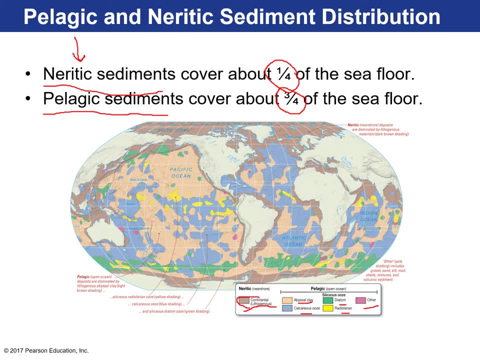 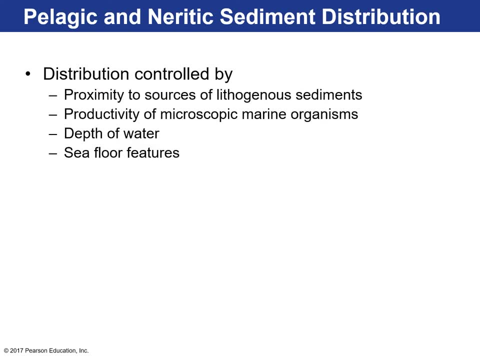 And if you see the continental lithogenous stuff really borders all the major land areas. You can see that there. So their distribution of those sediments are really obviously proximity to the sources of lithogenous sediments, the productivity of those marine organisms, How deep the water is, right, depending on which one of these will dissolve. 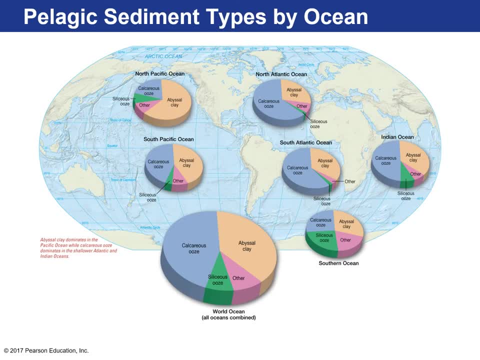 And some of the sea floor features. This is all the major oceans. This is the pelagic sediment type for all the major ocean basins. So if we look at the North Pacific Ocean, it's mostly made up of abyssal clay, some. 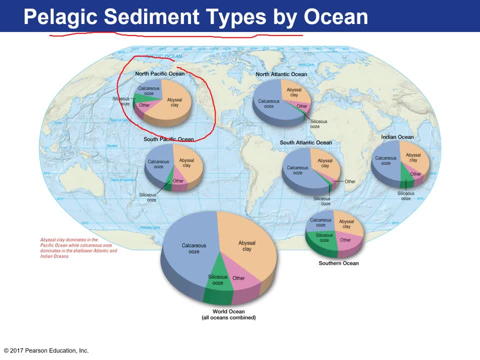 calcareous ooze and some siliceous oozes. The South Pacific has more calcareous oozes- Okay- And less abyssal clay. If we go to the world ocean average, this is the breakdown in pelagic sediment. 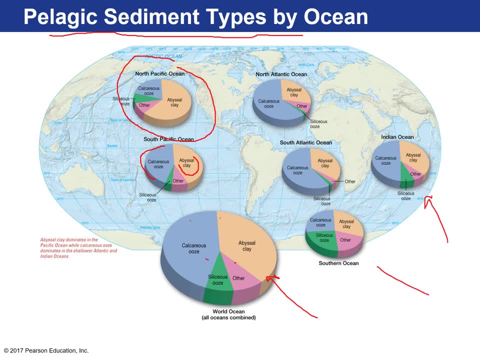 Okay, And these are all the breakdowns of the different oceans. You know there's some differences. Siliceous oozes aren't really found in the Atlantic as much as in other places In the Southern Ocean. you find a big proportion of siliceous oozes there. 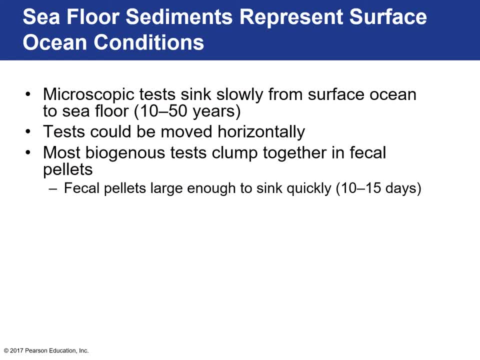 Okay, But a big question is like: how do we know that sea floor sediment represents? How do we know that these microscopic organisms, when they die their shells make it to the places directly above where they lived? I mean, if clay is taking 50 years to settle through the ocean column, don't you think? 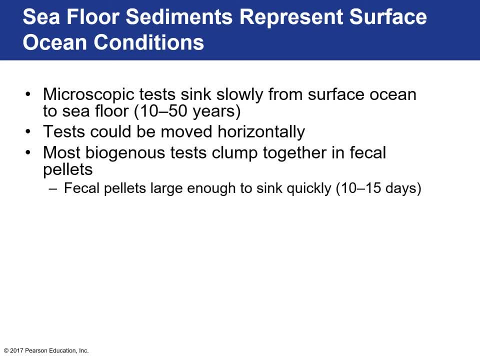 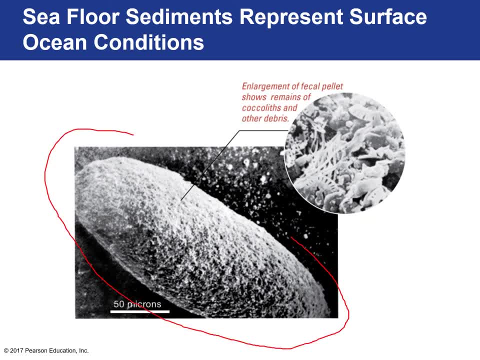 Okay, Okay. Here's a fecal pellet, guys, And this: if you cut this fecal pellet open and expose its contents, it'll be the dead remains of siliceous and calcareous organisms, and that's how they make it to the ocean floor. 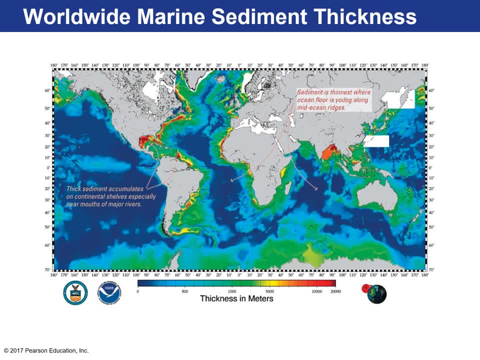 much quicker than suspension settling. Okay, If we look at worldwide marine thickness in terms of the amount of sediment that accumulates, so you can measure how much sediment is accumulated in areas, what you notice is most marine sediment has a lot of sediment. 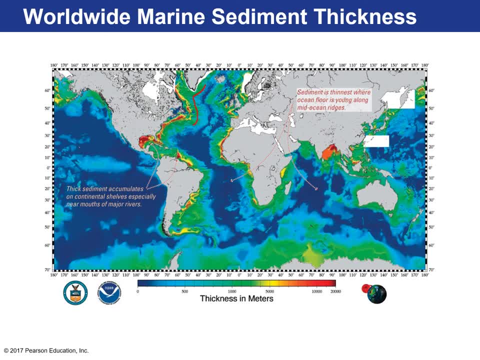 in terms of volume, is confined closest to the continents, which makes sense because, by volume, terriginous sediment is most abundant and those typically accumulate closest to their source. which are the continents Here? the Mississippi River, really, and the rivers that dump out into the Gulf, dump a. 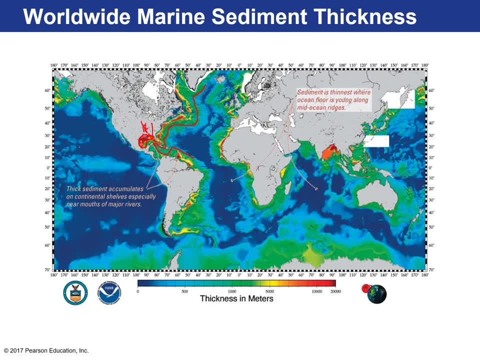 lot of sediment eroding from the Great Plains and the interior of the United States. The other major rivers that are kind of emptying out from eroded material from the Himalayas dump out into the Indian Ocean huge accumulations. Some of these accumulations are, if you see it's in red, that is, over 20 kilometers in. 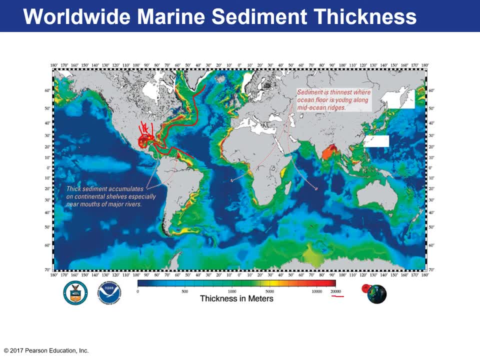 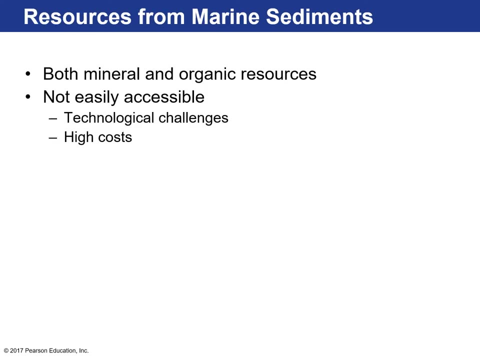 thickness. So 20 kilometers in thickness of sediment has accumulated on the ocean floor in some of these areas. Here's the deposits from the Orinoco River and the Amazon River. So yeah, so rivers really distribute a lot of sediment out into the open ocean. 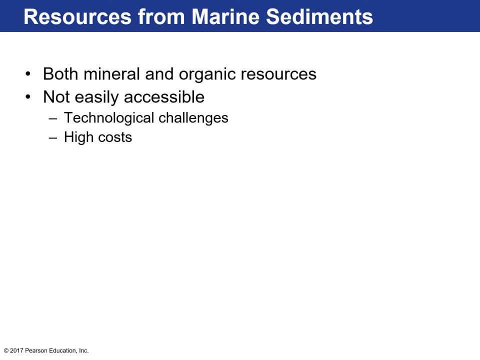 Okay, finally, just to kind of sum this up, I know you've been with me for a long time, so let's speed this up, I guess. but you can get a lot of resources from marine sediments. Both mineral and organic resources are important. 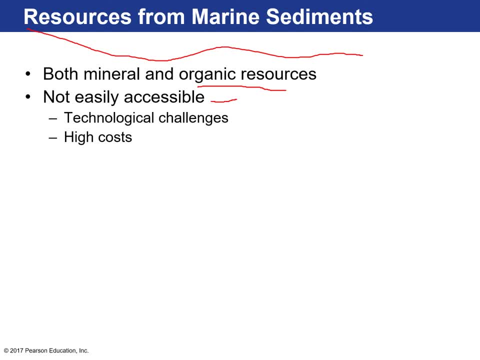 The problem with marine sediments is that they're not really easily accessible. No one's like: hey man, let's go out into the open ocean 300 miles off coast. There are a lot of costs and technological challenges with extracting those resources. 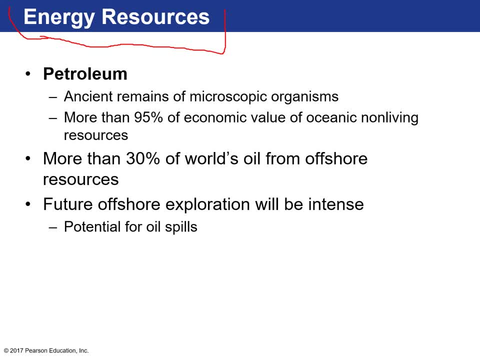 One of them that we do go out for a lot. Okay, One of the things we go out for a lot, especially on continental shells, is petroleum. Petroleum accumulates. remember we talked about diatoms, those single-celled algae that create their shells out of silica. 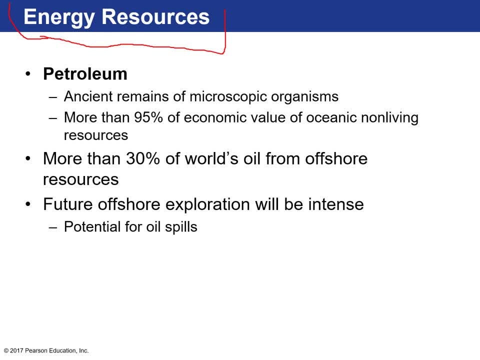 They often create a little droplet of oil inside of their shells because it makes them more buoyant to stay in the sunlit layers of the ocean. So when they die, that droplet of oil falls down with them and all their other dying compatriots. 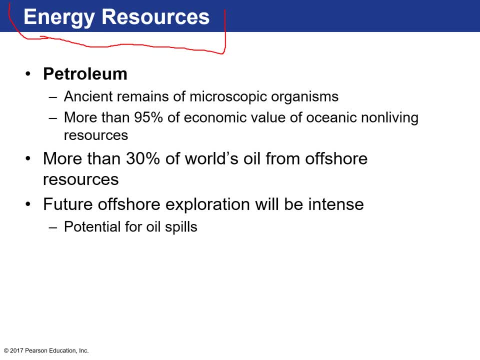 just raining down on the ocean floor That can accumulate and create petroleum that's found in the ocean. More than 30% of the world's oil comes today from offshore resources, And most of the land resources for oil have been found and used up or in the process of. 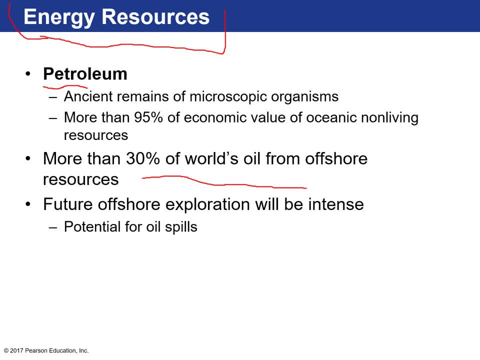 being used up. So future exploration will be intense in areas, Remote areas, Okay, Maybe off the coast of Alaska. Continental shells off a lot of our different continental margins So that leads to a lot of potential for oil spills, because that's happened and continues. 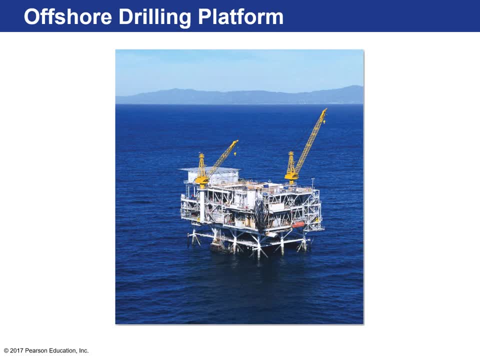 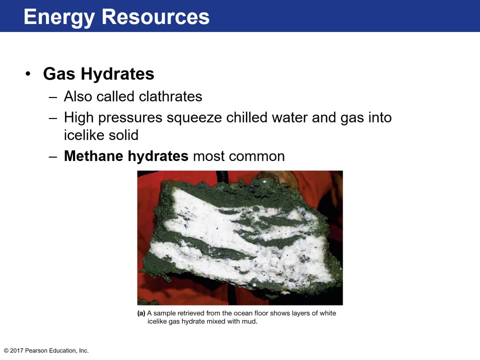 to happen. Okay, So here's an offshore drilling platform. This is what is built- to access those petroleum reserves that are in ocean sediment. Okay, Another interesting one are gas hydrates. These are a lot of times they're sediment that accumulates close to continents but at 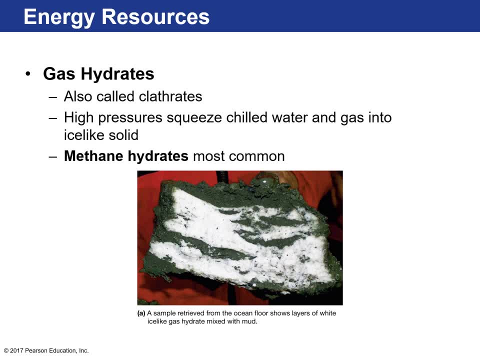 high latitudes, So it's really cold and under a lot of pressure, So that high pressure squeezes chilled water and methane gas and a lot of other gases into an ice, And so the most common gas is methane. Okay, So there's a lot of methane trapped and a lot of marine sediment in these specific environments. 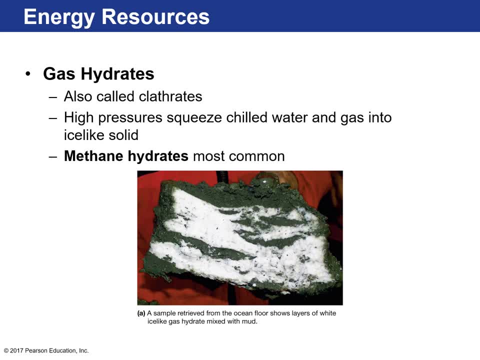 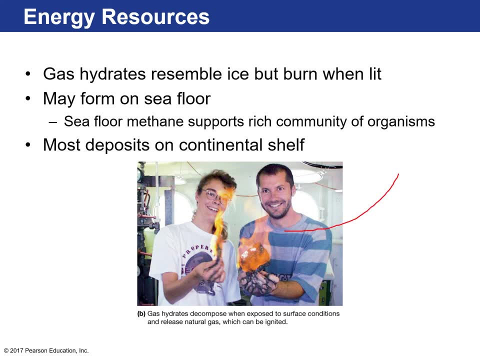 And when you drill them up or collect that sediment, you can- essentially because they're made of gas- you can- light them on fire. Look at these guys. they've grabbed some ocean sediment and lit it on fire. Ice hydrates, because they're made of ice under surface conditions like they're on. 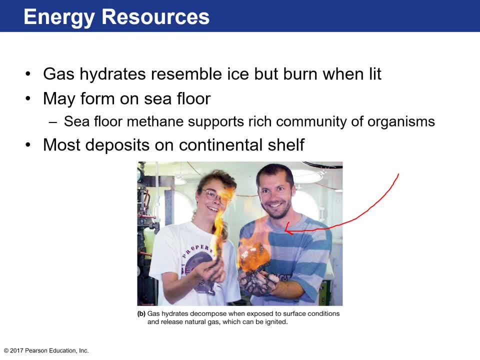 this boat. They're made to volatilize and evaporate into the air, so that's why you can light it on fire. So they're very unstable once you bring it onto surface conditions. So this: we mostly find those deposits on continental shelves. 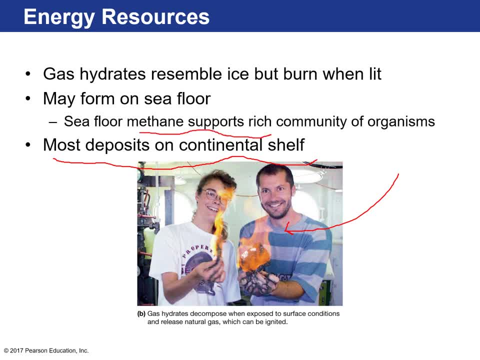 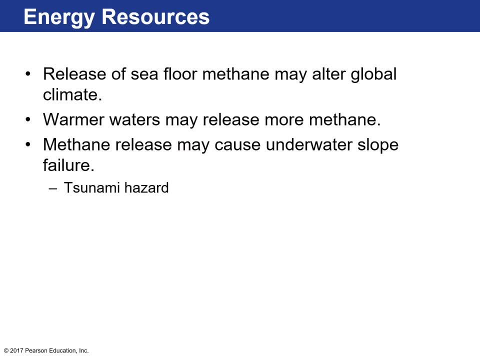 And, in fact, on the sea floor, that methane supports a really rich community of organisms that we're just kind of understanding today. Okay, So The reason why this is a potentially important resource is that we can use methane to create energy, essentially. 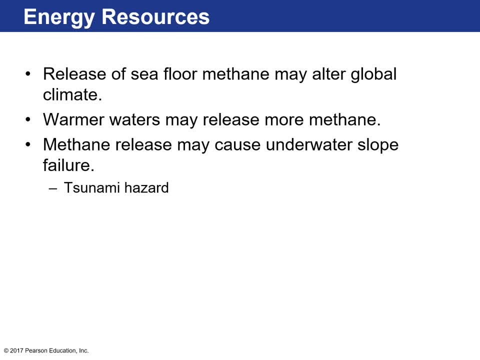 The problem is methane is a greenhouse gas, and the extraction methods for this ice haven't been perfected, and we don't really know how it affects the local sea floor communities that depend on that methane, And so it could be a really dirty business, And 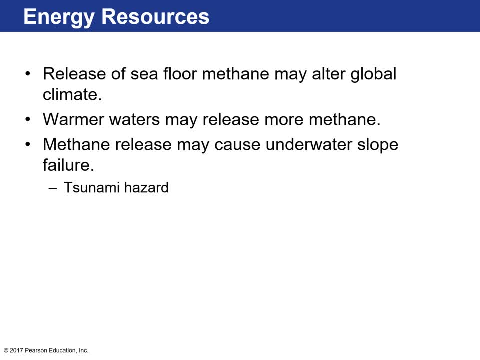 A lot of scientists are actually worried with the warming oceans. that warmer, deeper ocean waters could actually melt a lot of these ice hydrates and then it'll release a lot of methane from the ocean and into the atmosphere, which is a greenhouse gas, and then kind of 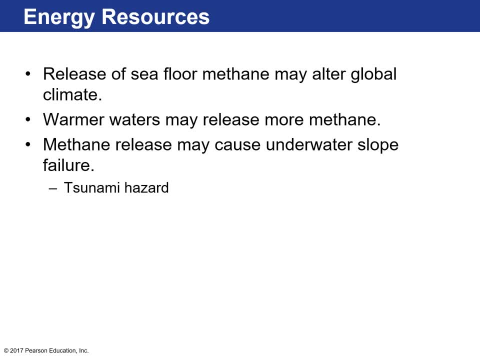 accelerate the global warming process. And also, if this were, if all that methane was were to be released in one kind of catastrophic- you know catastrophe- It could generate an incredible tsunami hazard as well, because it'll create an underwater slope failure. 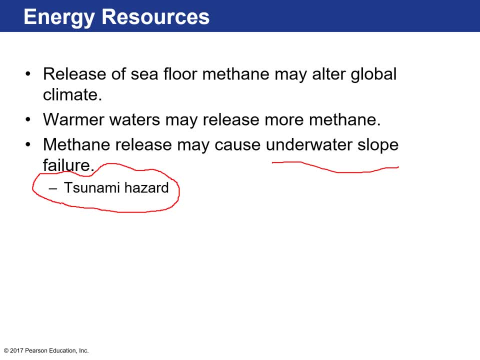 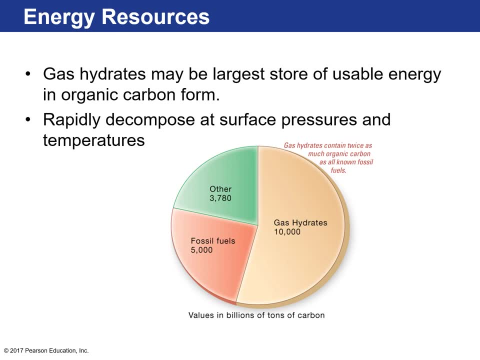 A lot of sediment will then kind of, under the force of gravity, move down towards the abyssal plain and cause a tsunami. So those hydrates: they may be the largest store of usable energy, but they rapidly decompose and they're hard to extract. 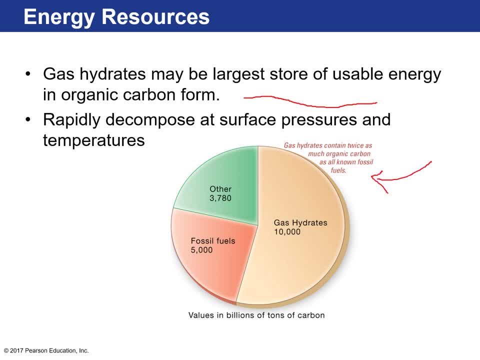 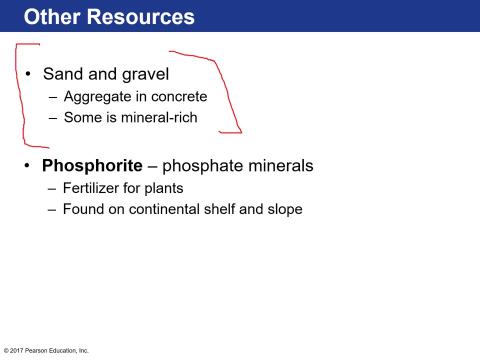 And we don't really know the effects of that extraction. So I mean it's not really a great resource that we could use right now. Other resources we use for ocean sediment, sand and gravel. We use a lot of sand and gravel in construction practices and creating cement. 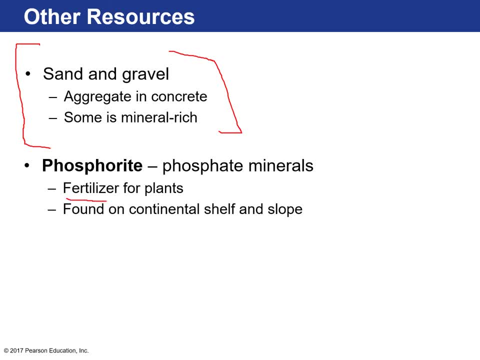 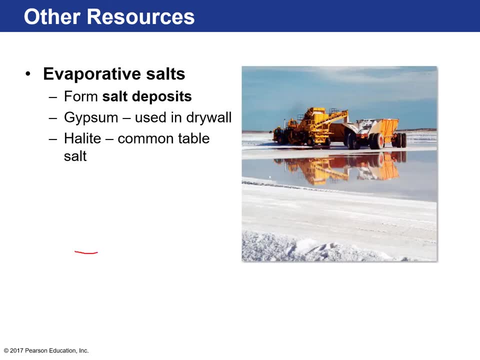 Phosphor deposits we use for fertilizer for plants, And so we typically find these on continental shelves and slopes, areas of high biological activity. Evaporite- evaporites we use, you know, to season our food. gypsums used in drywall. 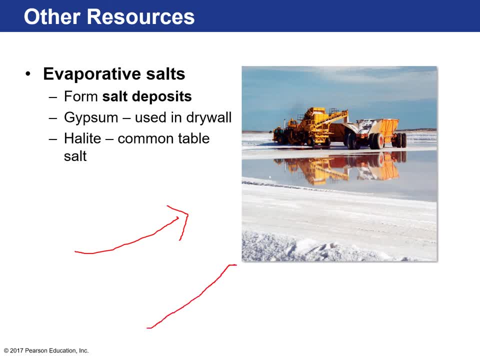 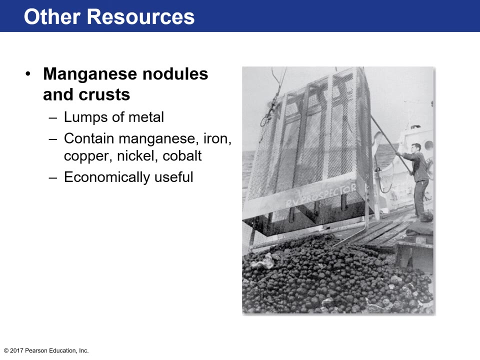 So a lot of places that were once covered by oceans- at least shallow oceans- have since evaporated away. We mine that stuff for our everyday use. Manganese nodules were also considered something to be mined, although it really depends on the price of those metals. 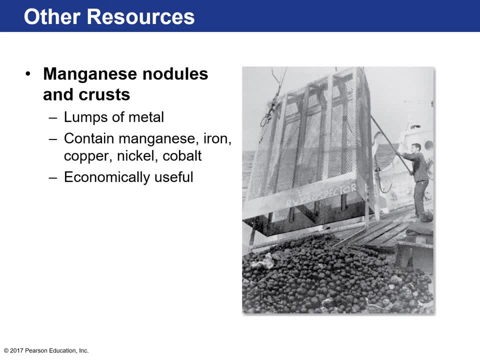 These nodules contain iron, copper, nickel and cobalt, which are all economically useful metals, But the prices so far for these metals have still been low- low enough to not make it really economically viable to go out into the middle of the ocean and disturb all the 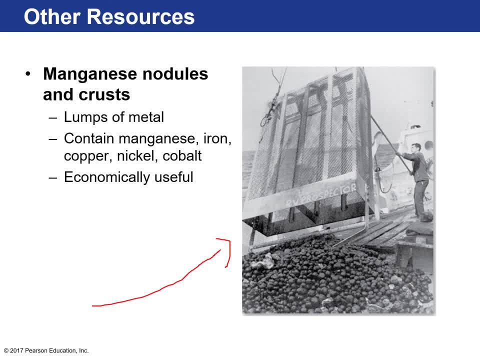 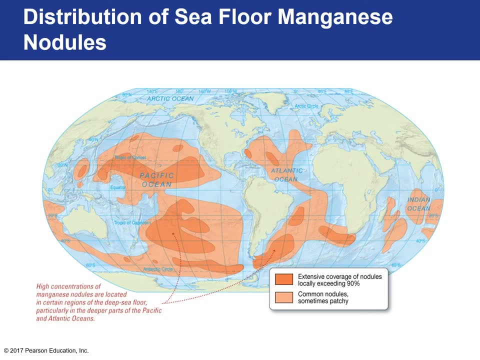 sediment to pick up these kind of baseball-sized manganese nodules. Here are the distribution of those manganese nodules. Okay, So in some cases, in some areas, interestingly enough, they exceed 90%, so they're more dense areas. So a lot of them are found in the Pacific Ocean. 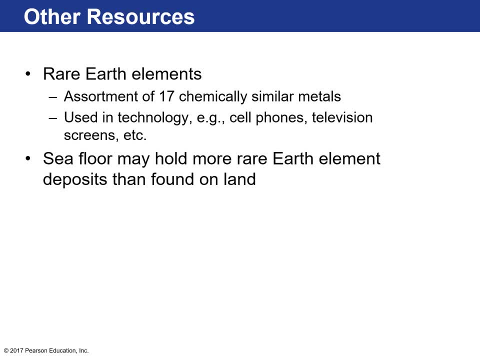 All right. and then, lastly, rare earth elements have become increasingly important because they're these metals that are not too abundant in a lot of different earth materials, but we use them in a lot of modern day technologies like cell phones and television screens.